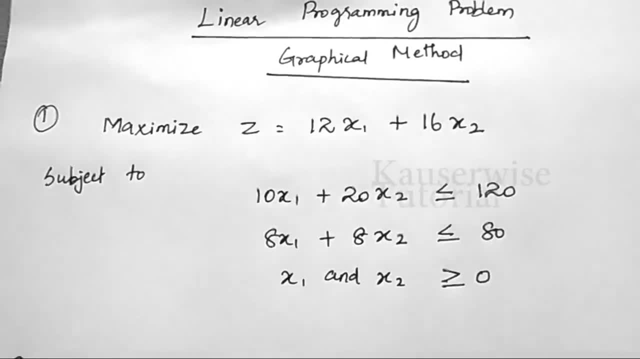 So, for example, we have LPP. So, for example, we have LPP. So, for example, we have LPP. So, for example, graphical method, simplex method, dual simplex method, big M method. So these are the different methods are available. 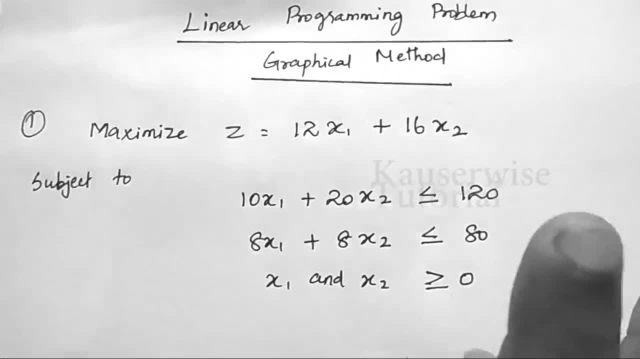 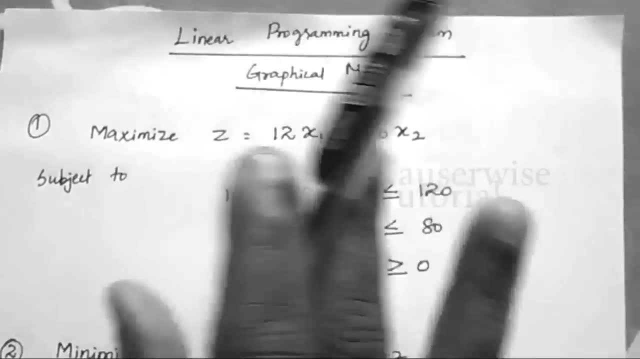 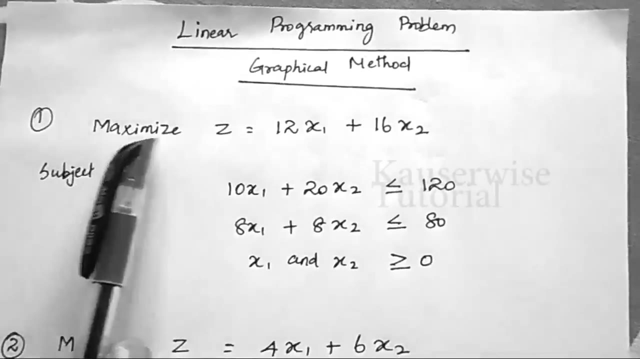 But the graphical method is applicable only when we have only two variables. If we have more than two variable means the graphical method is not suitable. So here I am going to explain three different models of graphical method. The first one is maximization problem. 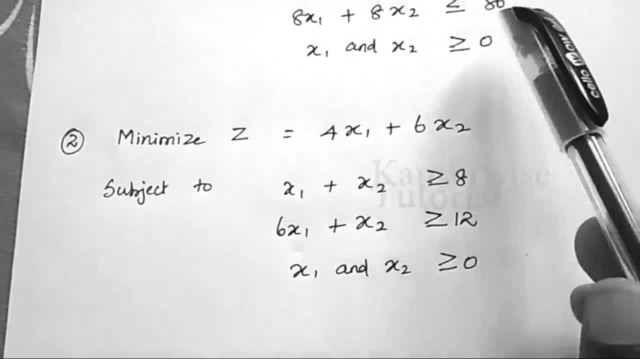 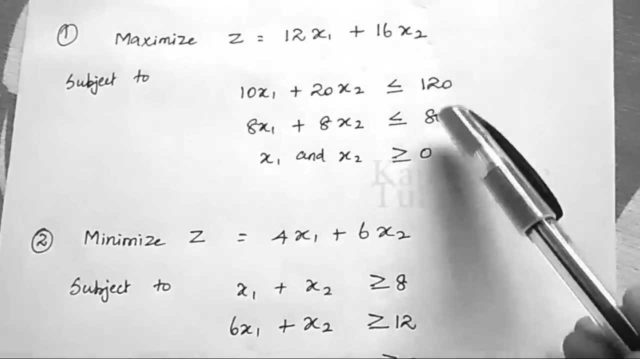 And second one is minimization problem. But in the first two methods we have two constraints. So this is the objective function subject to two constraints are given in the first problem. The second problem also same thing, But the first one is maximization problem. 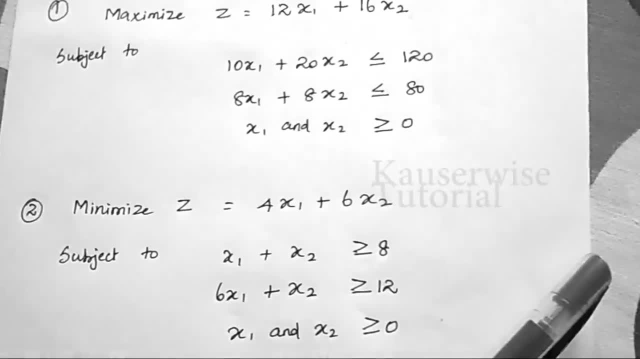 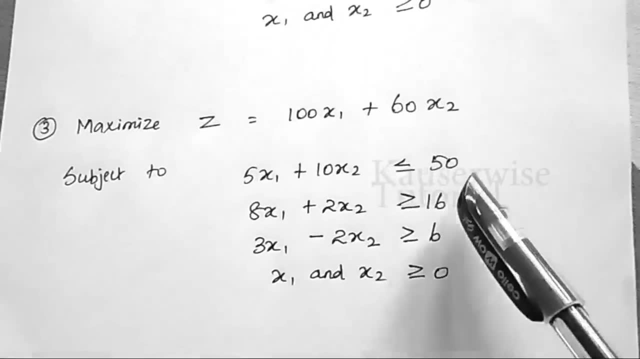 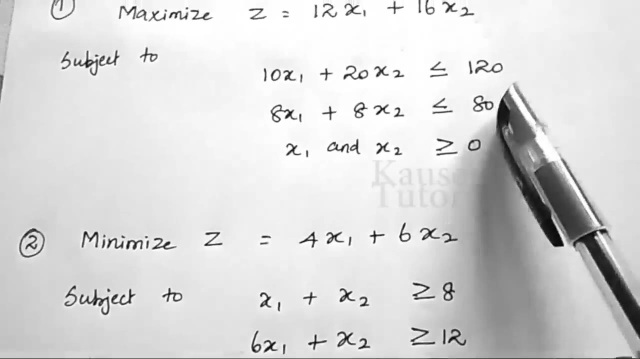 And second one for minimization problem. So I am going to explain two different models: Maximization model and minimization model, And the third one is maximization. But here we have three constraints. In the above two Problems we have only two constraints. 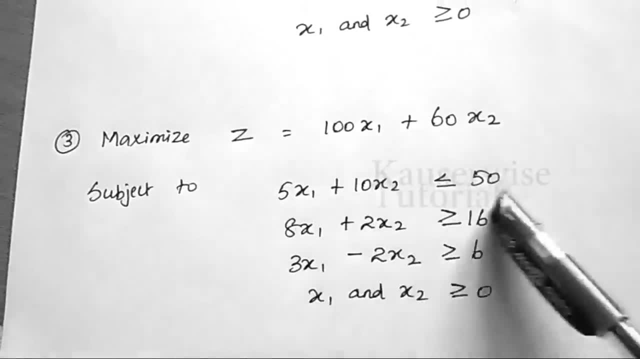 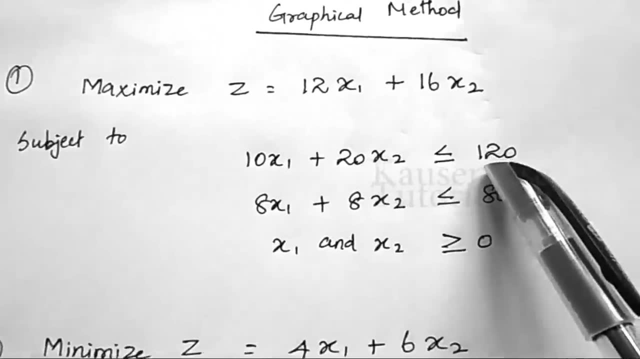 But in the third problem we have three constraints. So constraints means three equations are there. So here I am going to explain three things. In the first video I am going to explain the first one. The remaining, second and third, we will see in the separate video. 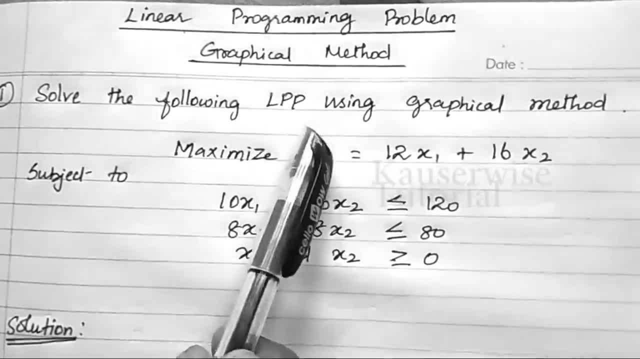 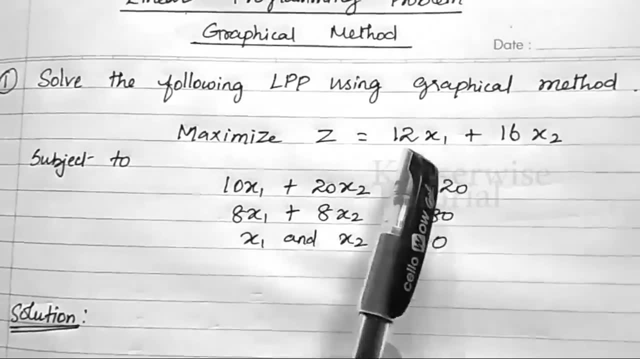 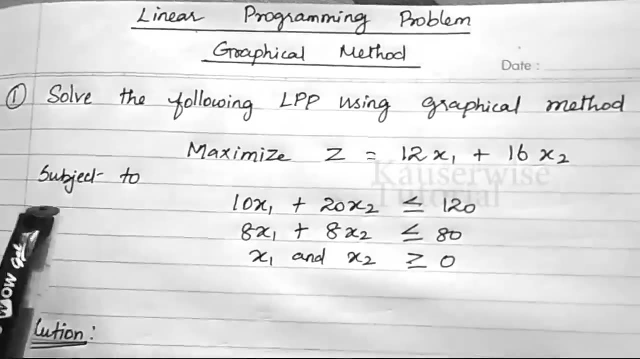 Let us see the first problem. See solve the following LPP using graphical method. This is a problem. Okay, maximize z is equal to 12x One plus 16x2.. This is the objective function of the problem, subject to two constraints are given. 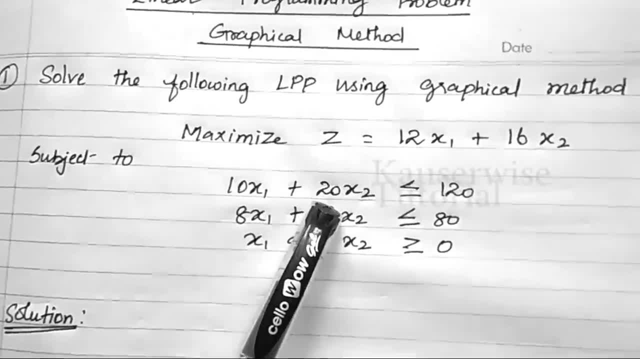 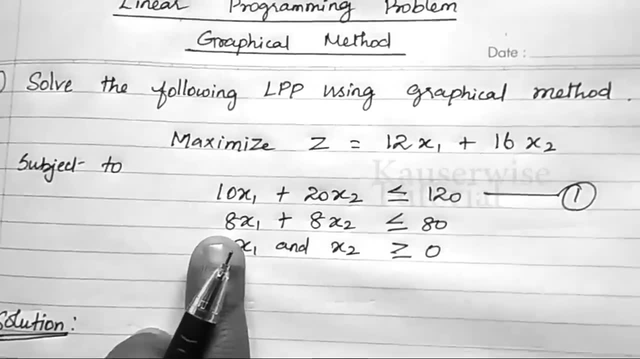 First one: 10x1 plus 20x2 less than or equal to 120.. This is the first constraint. And second constraint is 8x1 plus 8x2 less than or equal to 80.. So now we have two constraints. 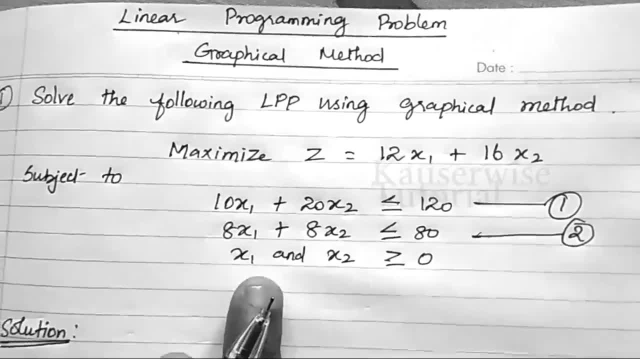 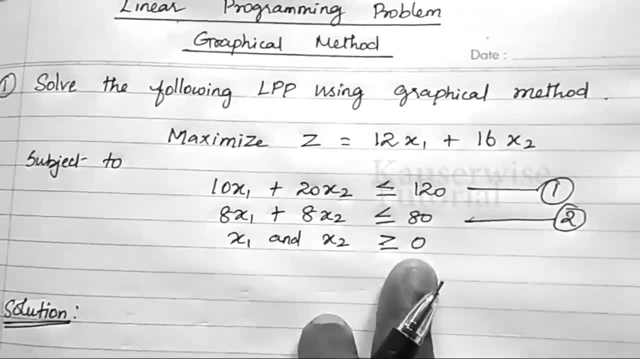 Our objective function is maximization problem. Okay, You need to find the value for x1 and x2.. The value should be greater than or equal to 0. Which means positive value. only Greater than or equal to 0 means 0 or more than 0.. 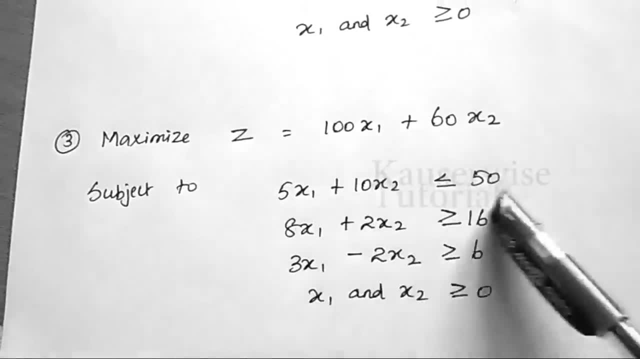 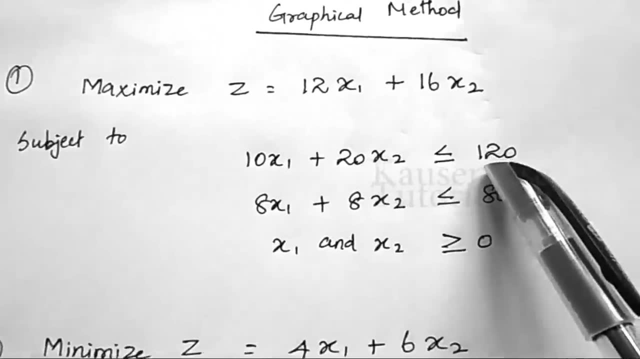 But in the third problem we have three constraints. So constraints means three equations are there. So here I am going to explain three things. In the first video I am going to explain the first one. The remaining, second and third, we will see in the separate video. 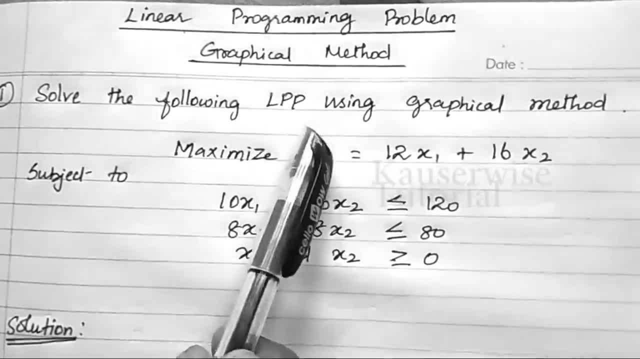 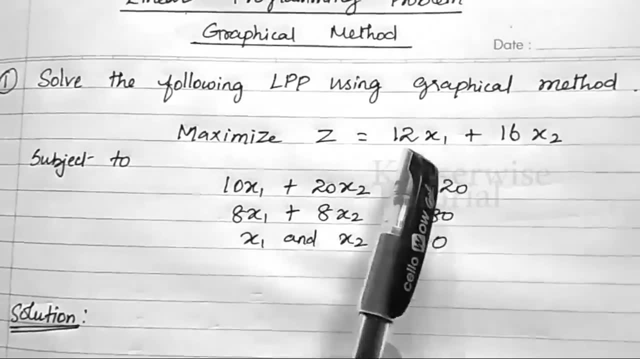 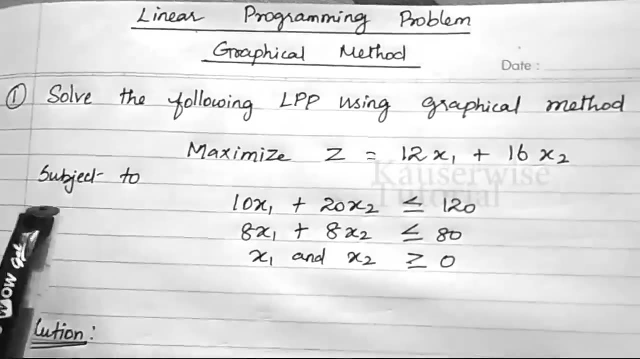 Let us see the first problem. See solve the following LPP using graphical method. This is a problem. Okay, maximize z is equal to 12x One plus 16x2.. This is the objective function of the problem, subject to two constraints are given. 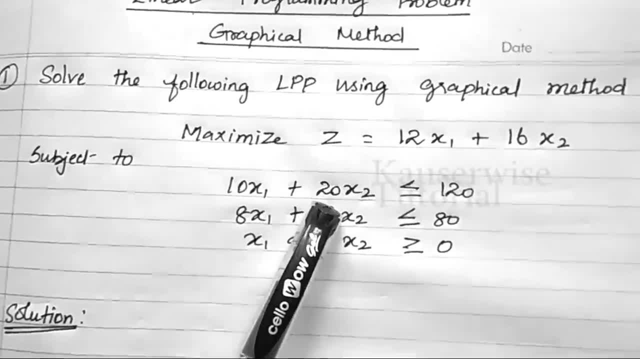 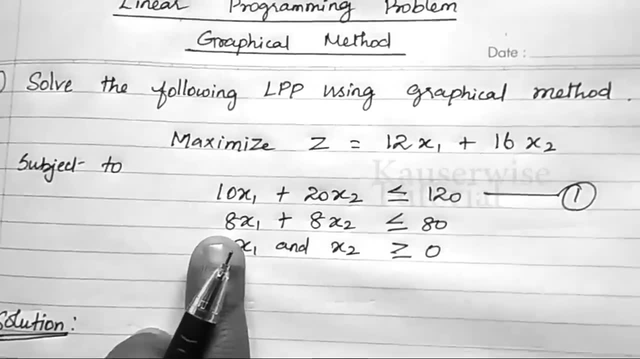 First one: 10x1 plus 20x2 less than or equal to 120.. This is the first constraint. And second constraint is 8x1 plus 8x2 less than or equal to 80.. So now we have two constraints. 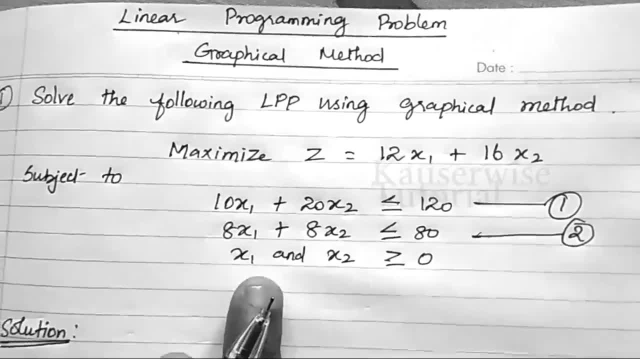 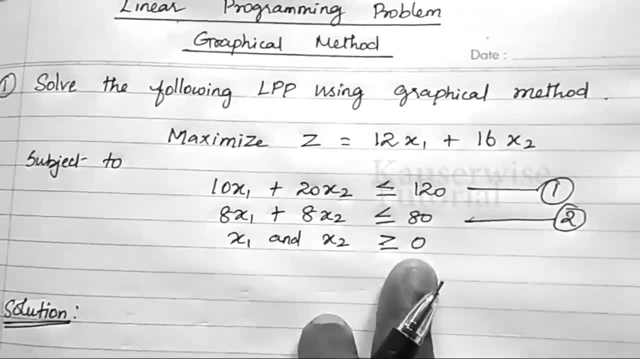 Our objective function is maximization problem. Okay, You need to find the value for x1 and x2.. The value should be greater than or equal to 0. Which means positive value. only Greater than or equal to 0 means 0 or more than 0.. 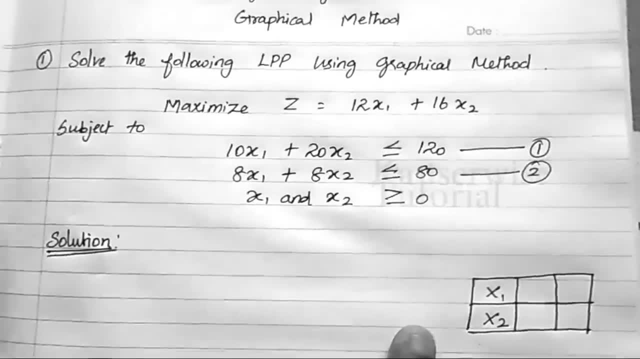 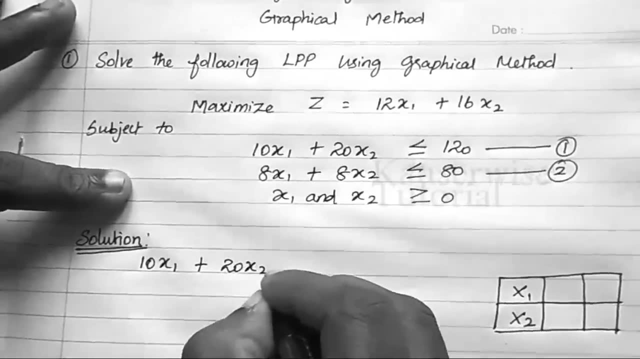 So first step is just convert the first constraint into an equation. So write the first one: 10x1 plus 20x2 is equal to 120.. So this is the first equation. So now we have to find the value. 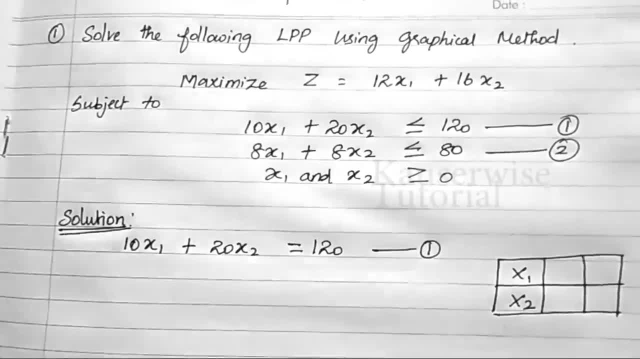 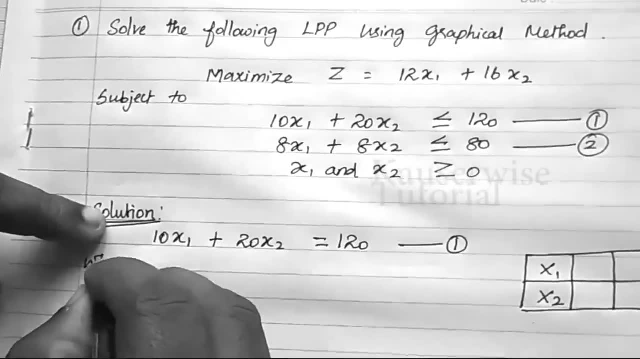 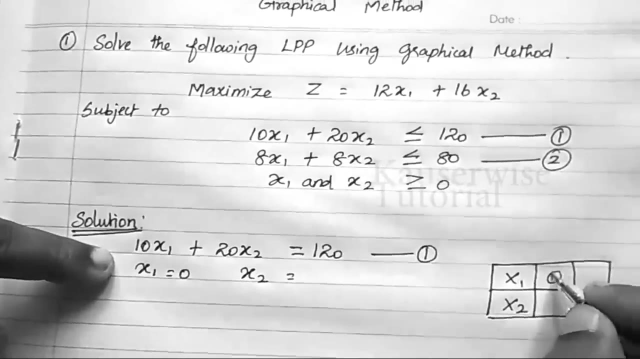 We need two points to plot in the graph sheet. Okay, So, first thing, you need to take x1 as 0.. See, when x1 is equal to 0,, what is the value for x2?? So, when x1 is 0,, what is the value for x2?? 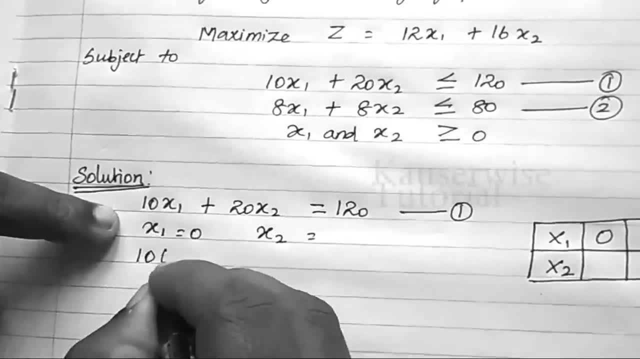 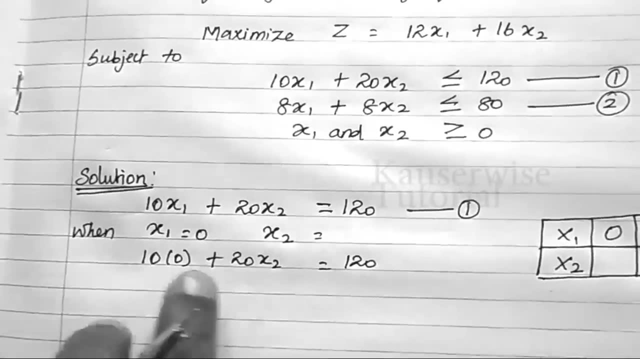 Let's apply this in the first equation: 10x1 is 0 plus 20x2 is equal to 120.. 10 into 0 is 0.. We have only 20x2.. So 20x2 is equal to 120.. 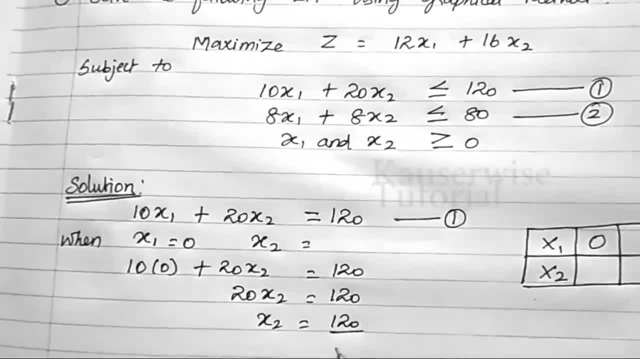 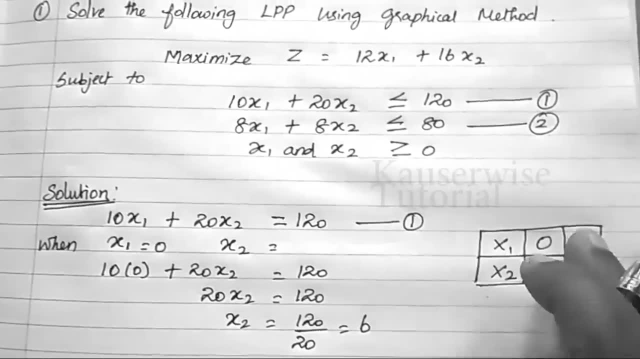 So x2 is equal to 120. divided by 20 is equal to 6.. So x2 value is 6.. When x1 is 0, x2 will be 6.. In the same way, now we have to consider x2 is equal to 0. 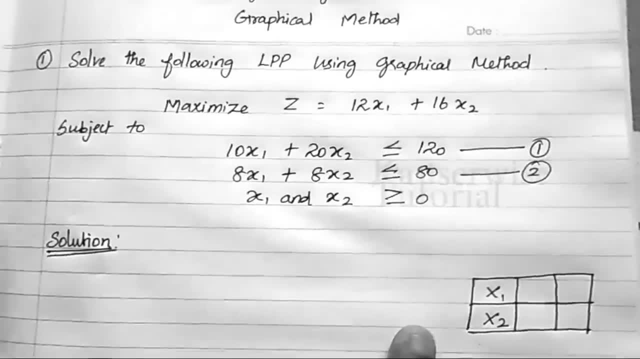 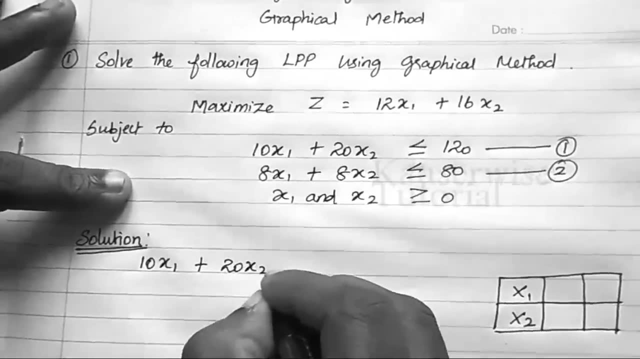 So first step is just convert the first constraint into an equation. So write the first one: 10x1 plus 20x2 is equal to 120.. So this is the first equation. So now we have to find the value. 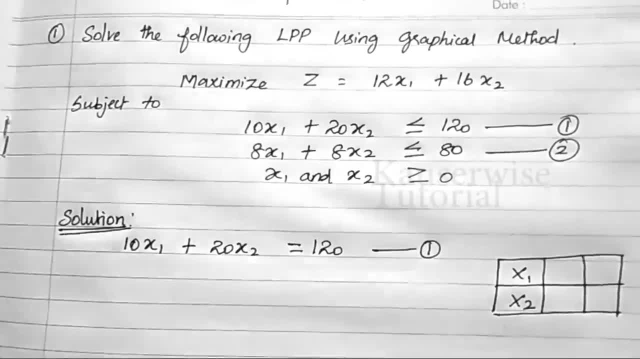 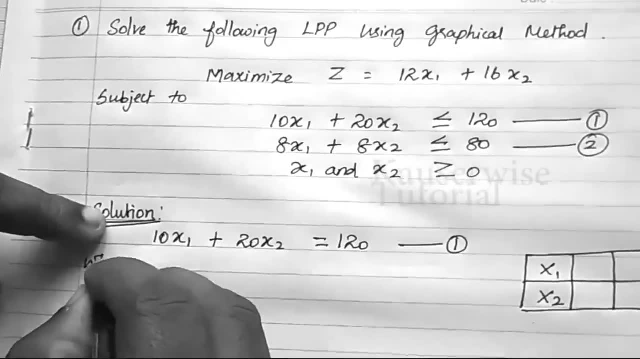 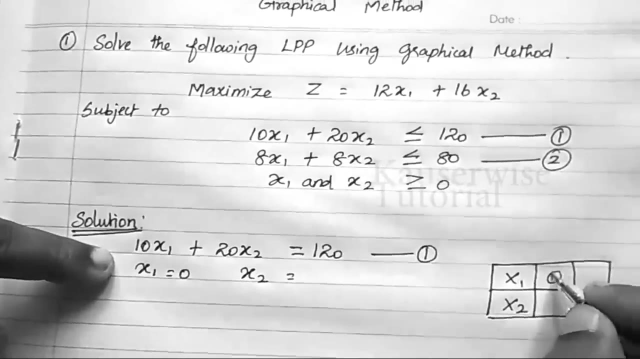 We need two points to plot in the graph sheet. Okay, So, first thing, you need to take x1 as 0.. See, when x1 is equal to 0,, what is the value for x2?? So, when x1 is 0,, what is the value for x2?? 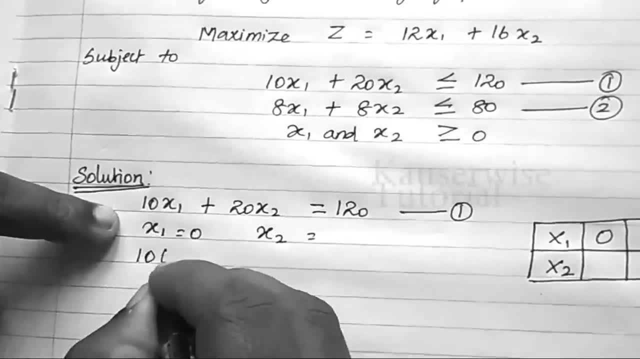 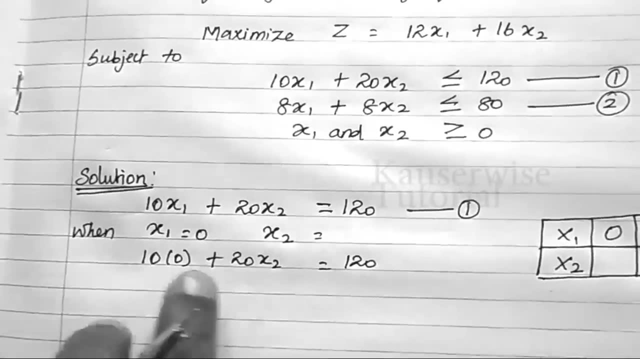 Let's apply this in the first equation: 10x1 is 0 plus 20x2 is equal to 120.. 10 into 0 is 0.. We have only 20x2.. So 20x2 is equal to 120.. 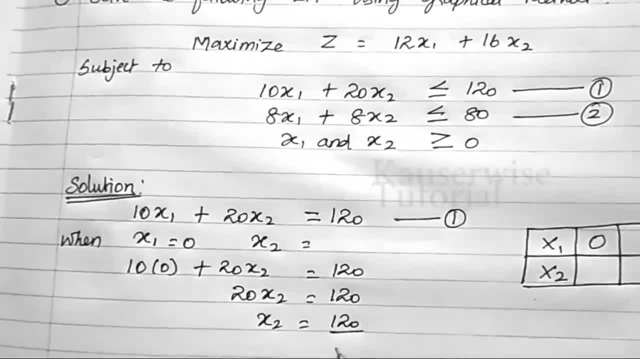 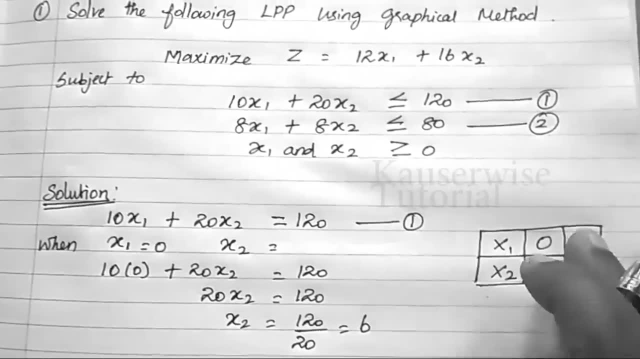 So x2 is equal to 120. divided by 20 is equal to 6.. So x2 value is 6.. When x1 is 0, x2 will be 6.. In the same way, now we have to consider x2 is equal to 0. 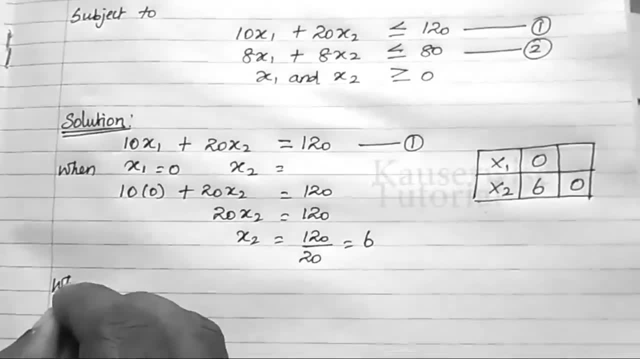 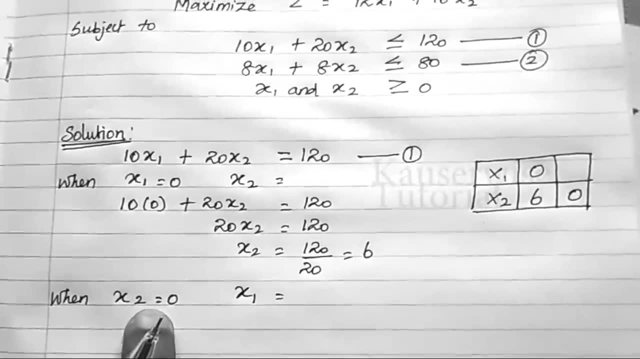 Then what is the value for x1?? When x2 is equal to 0,, what is the value for x2?? What is the value for x1?? Just apply this in the same equation: 10x1 plus 20x2 value is 0. 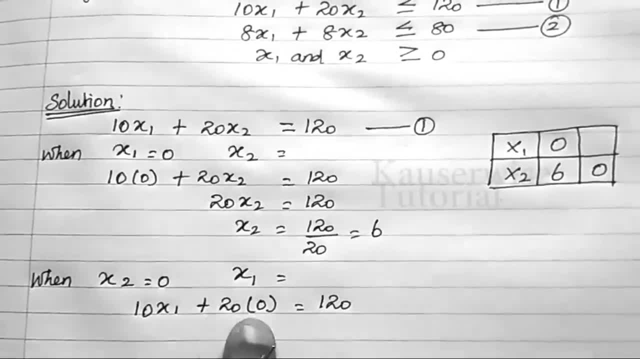 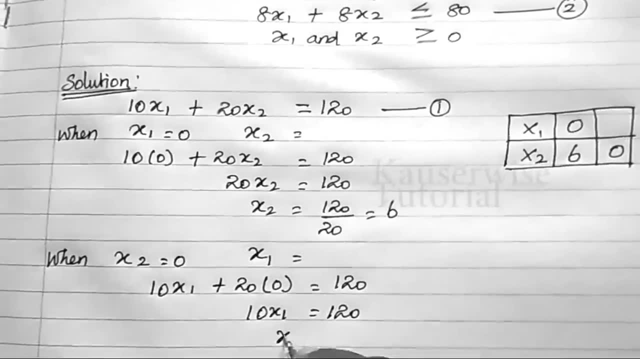 No, put 0 here 120.. So 20 into 0 is 0.. We have only 10x1.. So 10x1 is equal to 120.. x1 is equal to 120 divided by 10.. 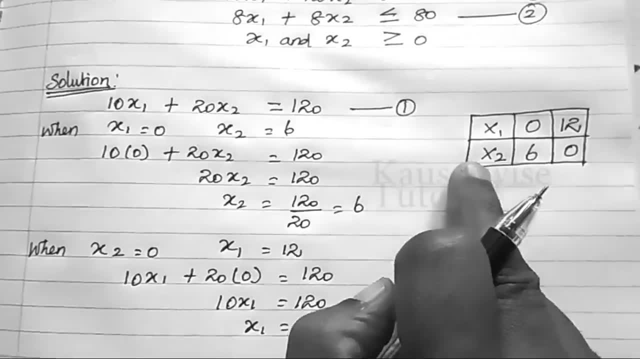 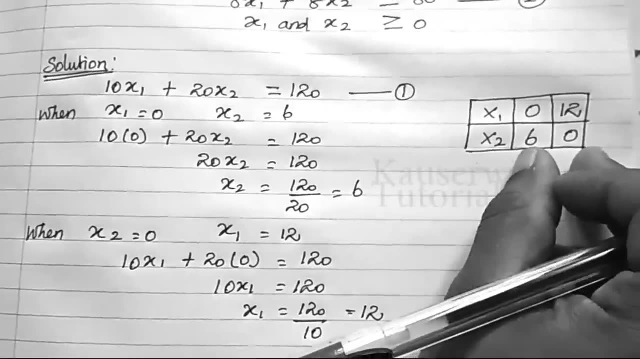 So x1 is equal to 12.. When x2 is equal to 0, x1 value will be 6.. x1 value will be 12.. So now we have got two points. With this you can plot into the graph sheet. 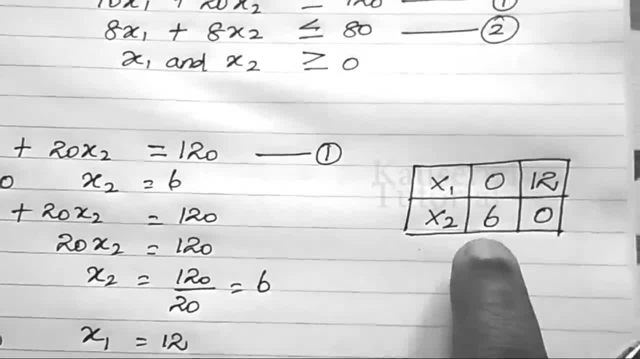 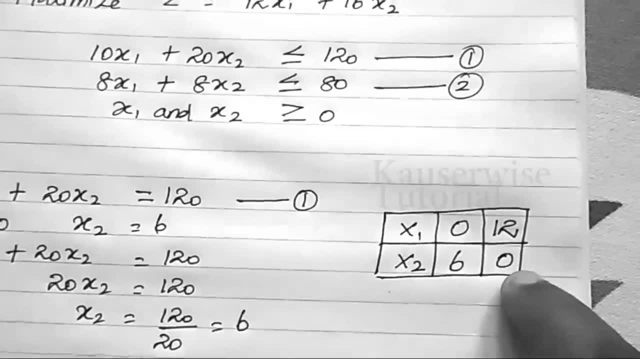 In order to draw a line, we need to have two points, Okay, first one is x1, 0, x2, 6.. This is the first point, And second point is x1, 12, x2, 0.. 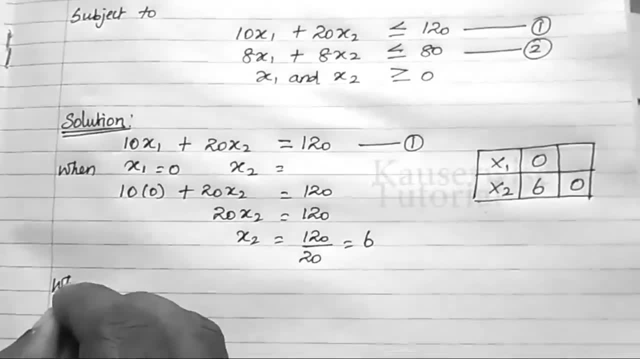 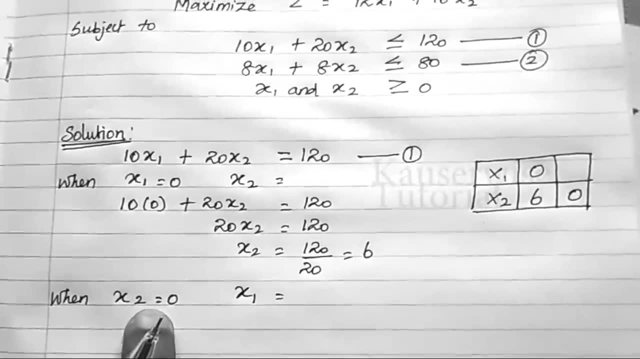 Then what is the value for x1?? When x2 is equal to 0,, what is the value for x2?? What is the value for x1?? Just apply this in the same equation: 10x1 plus 20x2 value is 0. 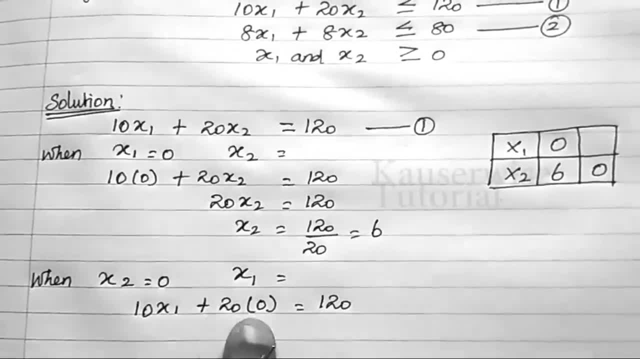 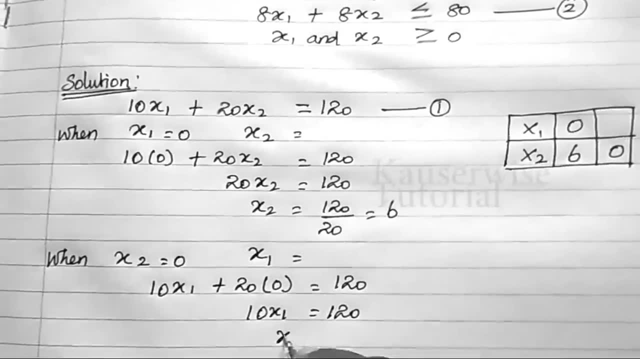 No, put 0 here 120.. So 20 into 0 is 0.. We have only 10x1.. So 10x1 is equal to 120.. x1 is equal to 120 divided by 10.. 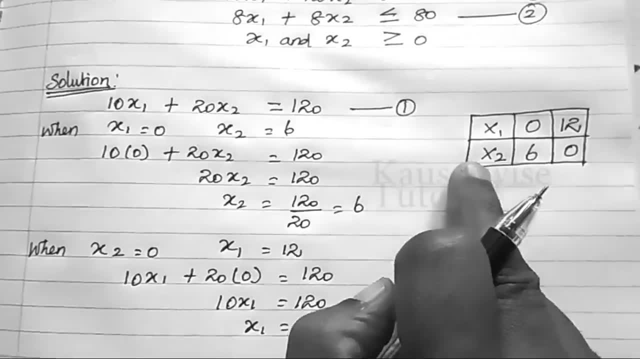 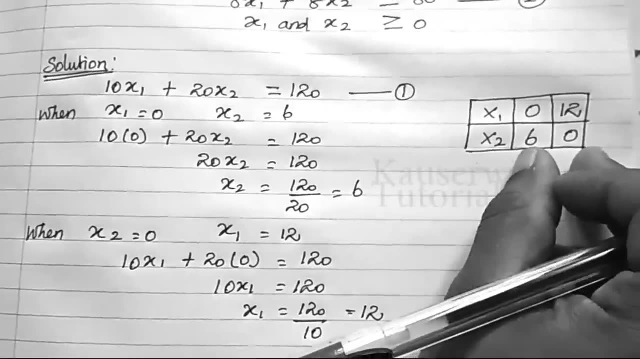 So x1 is equal to 12.. When x2 is equal to 0, x1 value will be 6.. x1 value will be 12.. So now we have got two points. With this you can plot into the graph sheet. 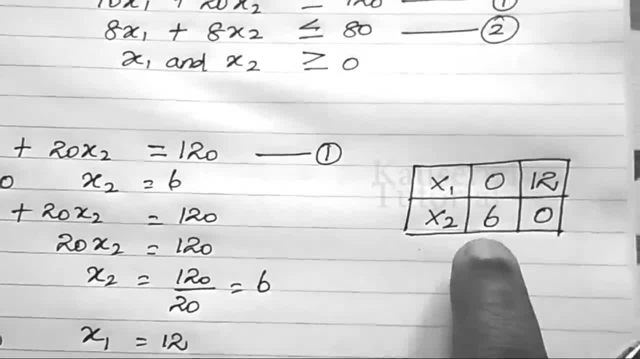 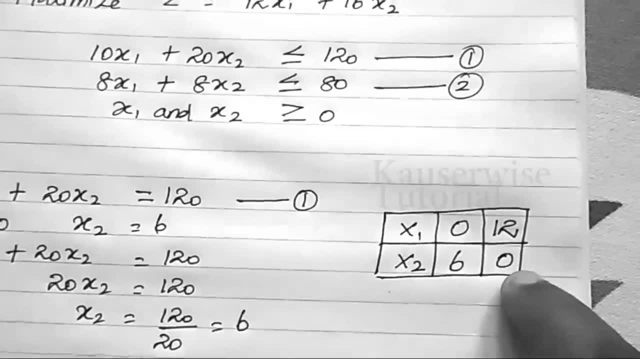 In order to draw a line, we need to have two points, Okay, first one is x1, 0, x2, 6.. This is the first point, And second point is x1, 12, x2, 0.. 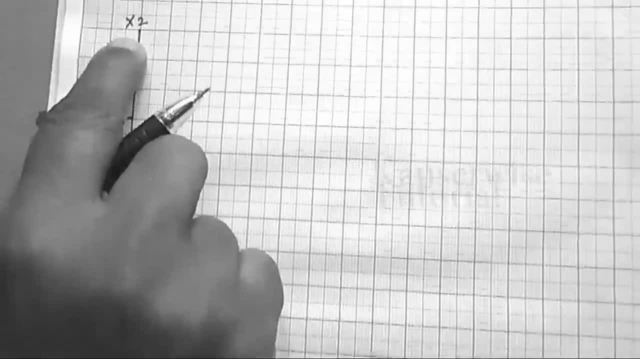 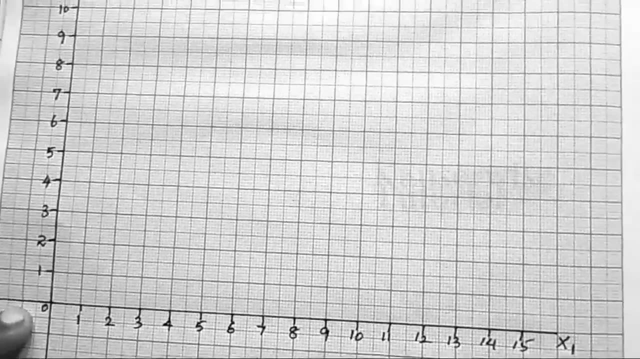 This axis x1 axis And this one is x2 axis. So plot the line First one: x1, 0, x2, 6.. x1, 0. 0, x2, 6.. 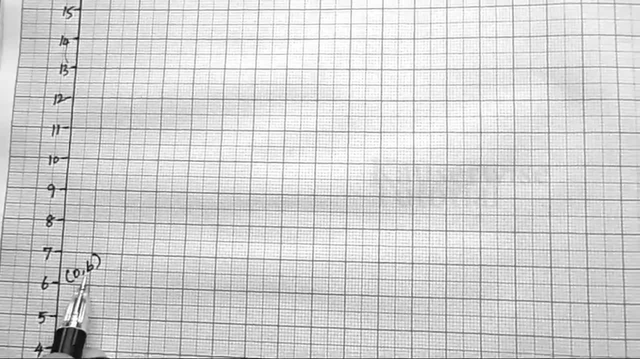 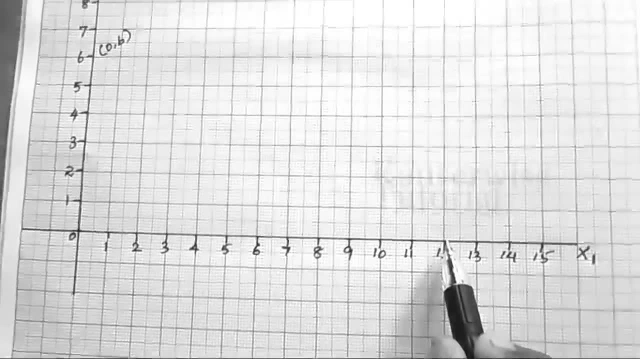 0, 6.. x1, 0, x2, 6.. Second point: x1, 12, x2, 0.. x1, 12, x2, 0.. So this is the point. 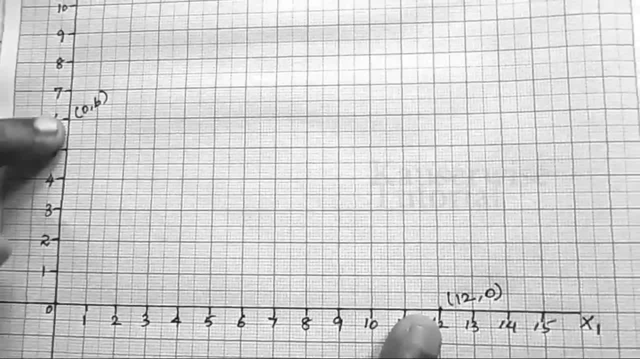 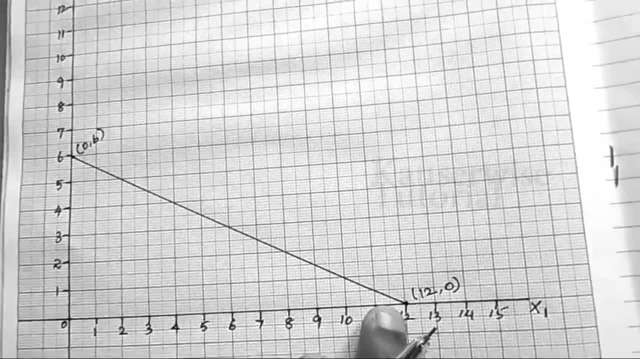 x1, 12, x2, 0.. We have got two points. Just join the two points to make a line. This line represents the first constraint. Now we have to find the second line. Okay, look at the problem. 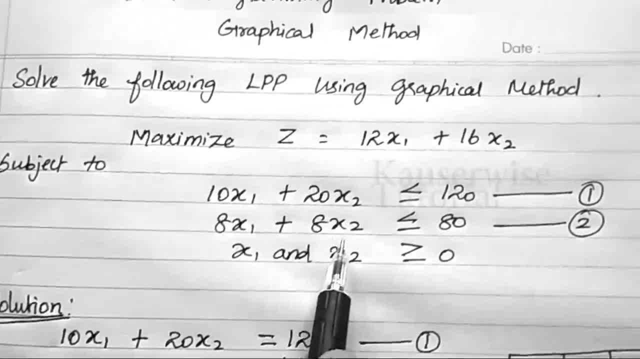 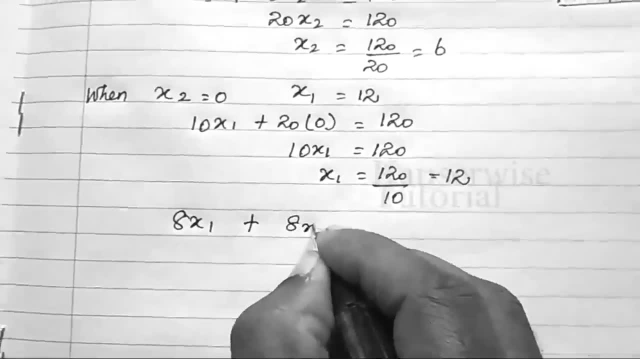 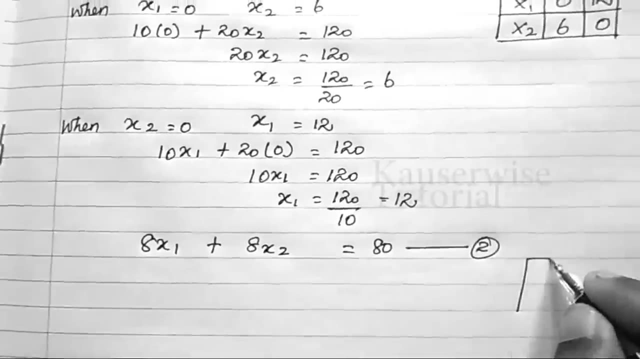 Look at the second constraint: 8x1 plus 8x2 less than or equal to 80.. Second equation: 8x1 plus 8x2 is equal to 80. So second equation: In the same way, we need to find the value for x1 and x2.. 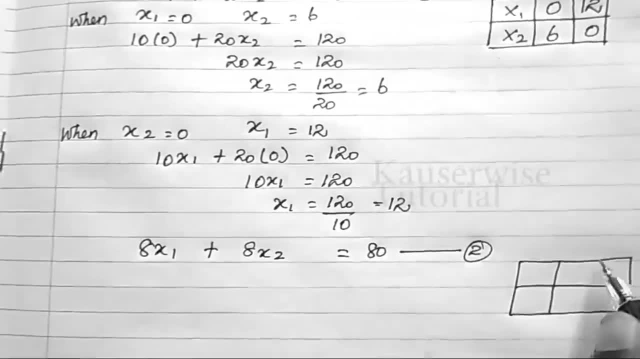 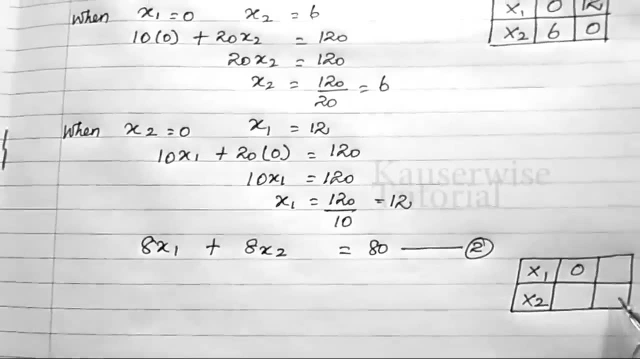 So, in order to draw a line, we need to have two points: x1, x2.. When x1 is 0,, what is the value for x2?? In the same way, when x2 is 0,, what is the value for x1?? 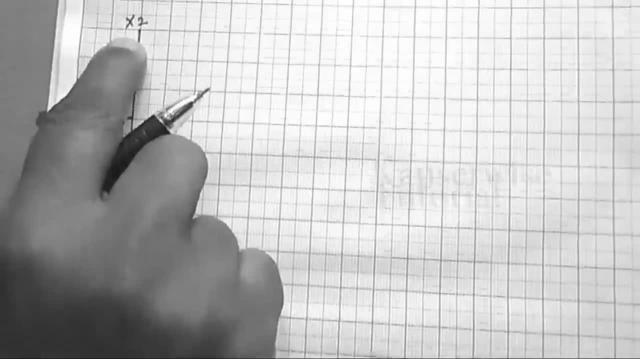 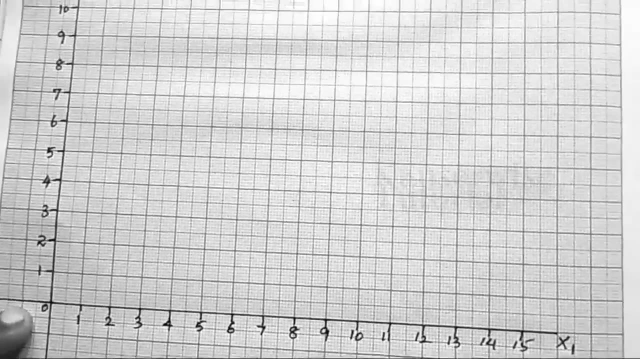 This axis x1 axis And this one is x2 axis. So plot the line First one: x1, 0, x2, 6.. x1, 0, x2, 6.. x2, 6, 0.. 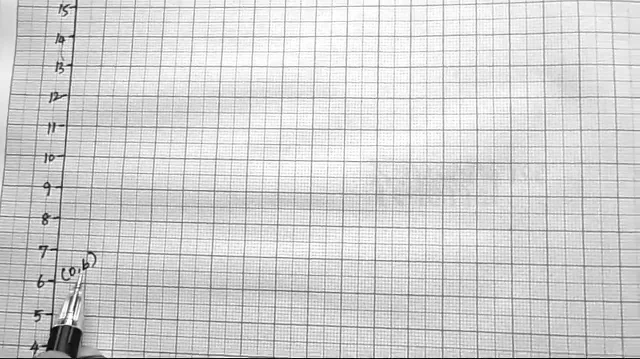 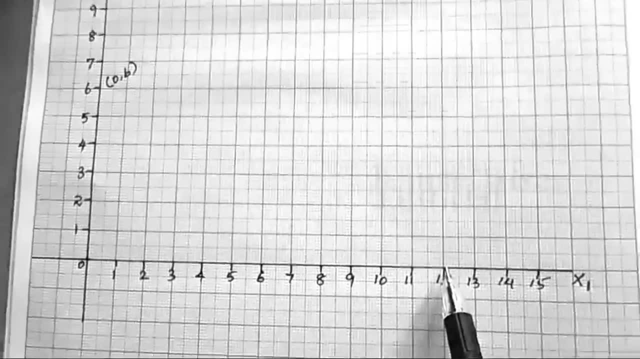 0, 6, 0.. x1, 0, x2, 6.. Second point: x1, 12, x2, 0.. x1, 12, x2, 0.. So this is the point. 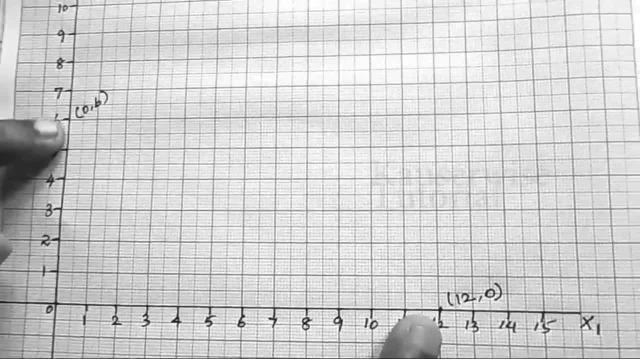 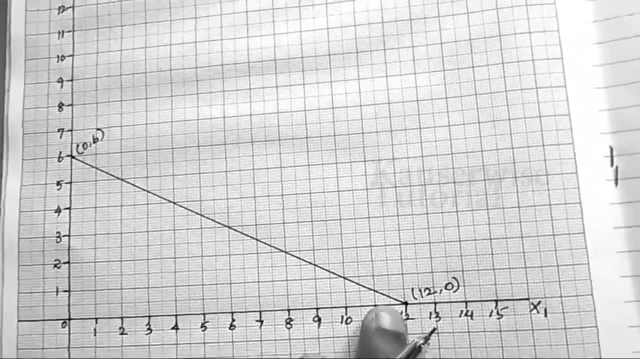 x1, 12, x2, 0.. We have got two points. Just join the two points to make a line. This line represents the first constraint. Now we have to find the second line. Okay, look at the problem. 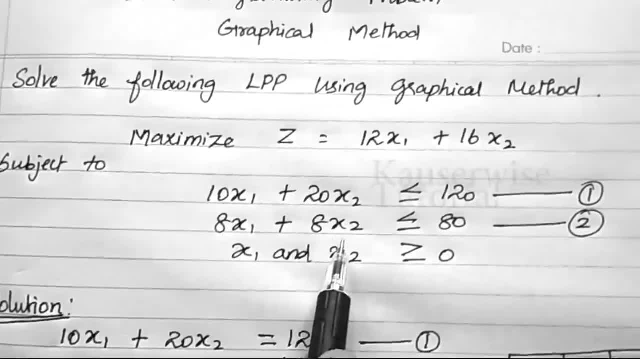 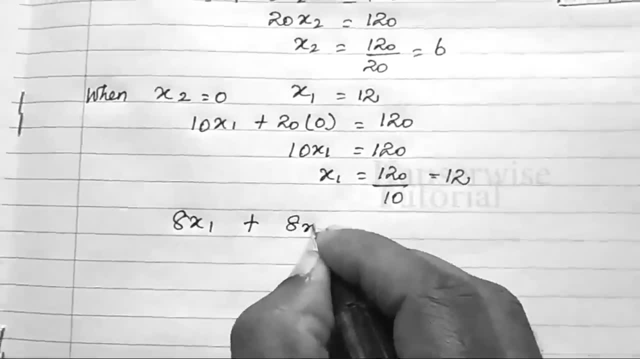 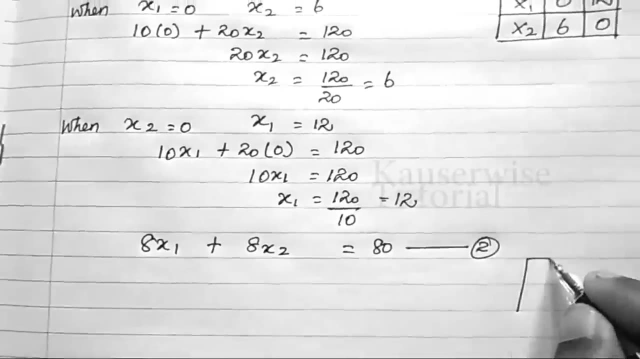 Look at the second constraint: 8x1 plus 8x2 less than or equal to 80.. Second equation: 8x1 plus 8x2 is equal to 80. So second equation: In the same way, we need to find the value for x1 and x2.. 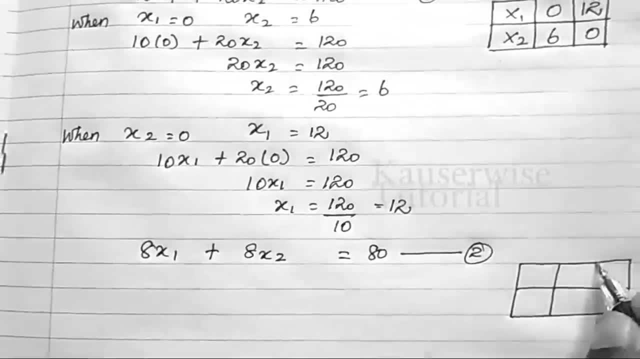 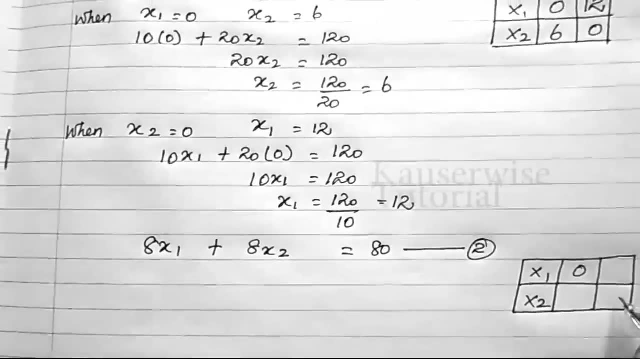 So, in order to draw a line, we need to have two points: x1, x2.. When x1 is 0,, what is the value for x2?? In the same way, when x2 is 0,, what is the value for x1?? 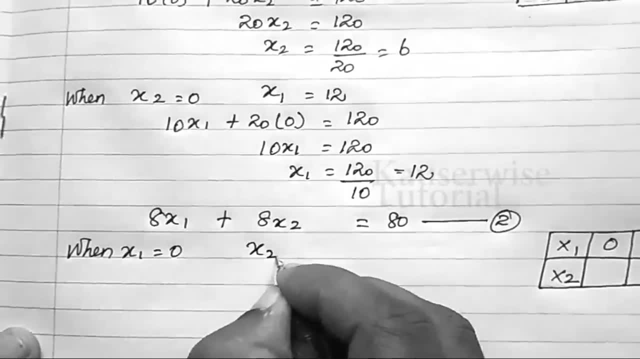 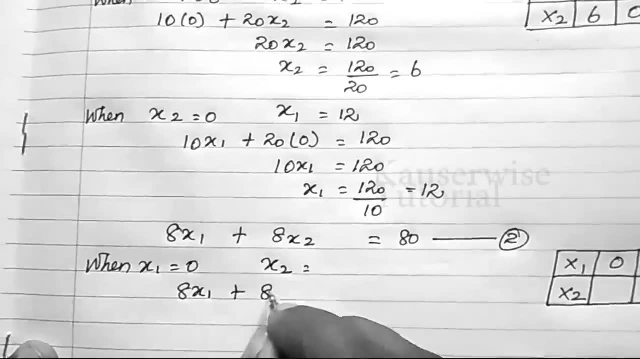 When x1 is equal to 0,, what is the value for x2?? Okay, just apply this in the equation 8x1, that is, 8x1 plus 8x2 is equal to 80.. No, So 8 into 0. 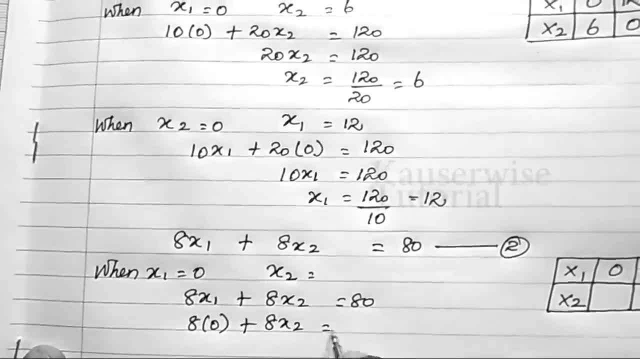 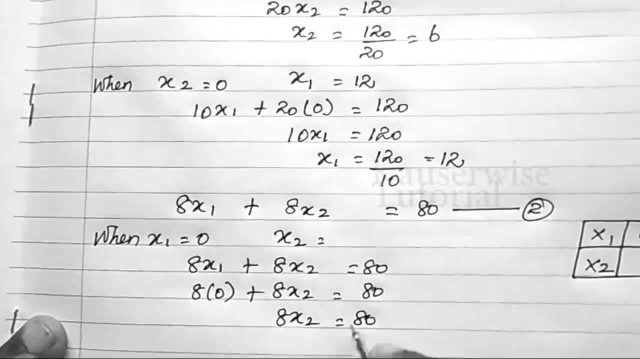 x1 value is 0.. No, No, Plus 8x2 is equal to 80.. 8 into 0 is 0.. We have only 8x2.. 8x2 is equal to 80.. So x2 is equal to 80 divided by 8.. 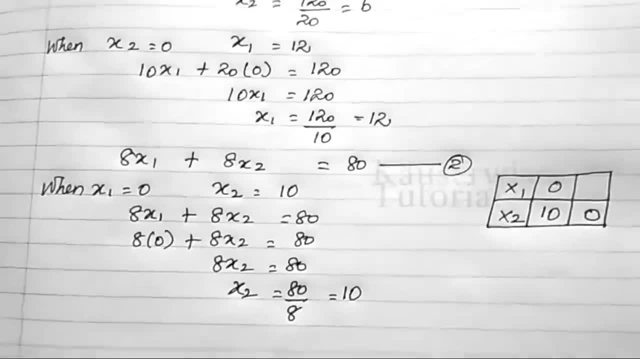 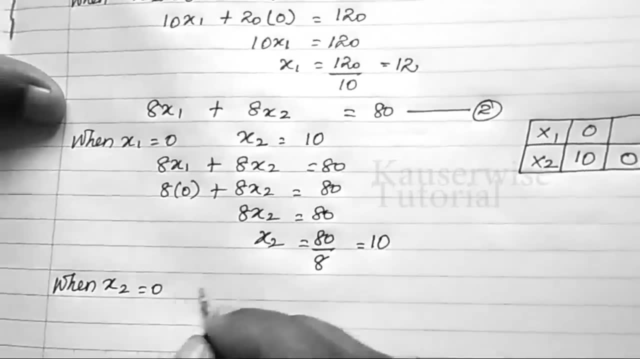 So what is the value? 10.. 10. In the same way, find the value for x1.. When x2 is equal to 0,, what is the value for x1?? What is the equation 8x1.? 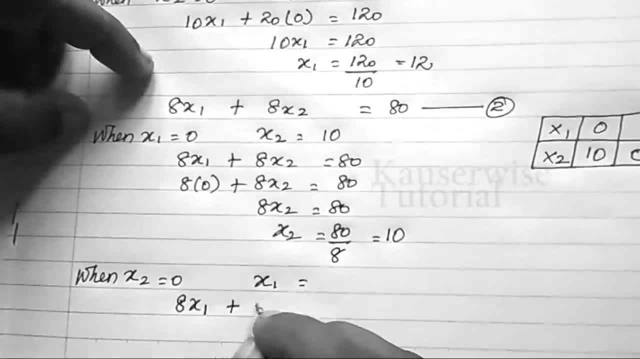 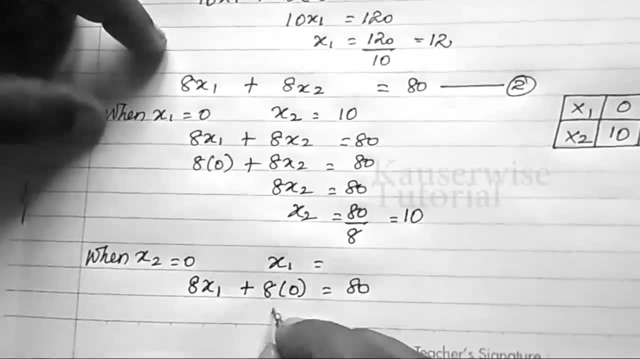 No, So 8x2.. 8x1 plus 8x2 value is 0, is equal to 80.. 8 into 0 is 0.. We have only 8x1.. 8x1 is equal to 80.. 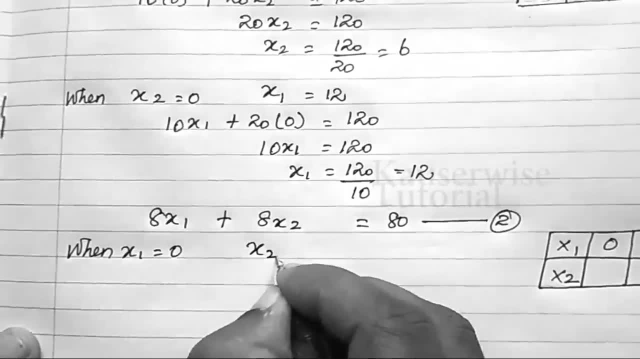 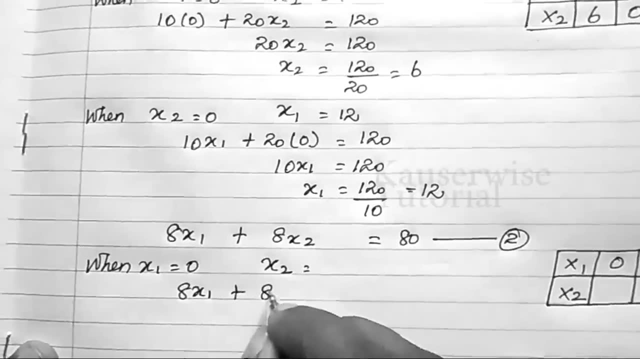 When x1 is equal to 0,, what is the value for x2?? Okay, just apply this on the equation 8x1, that is, 8x1 plus 8x2 is equal to 80.. No, So 8 into 0, x1 value is 0. 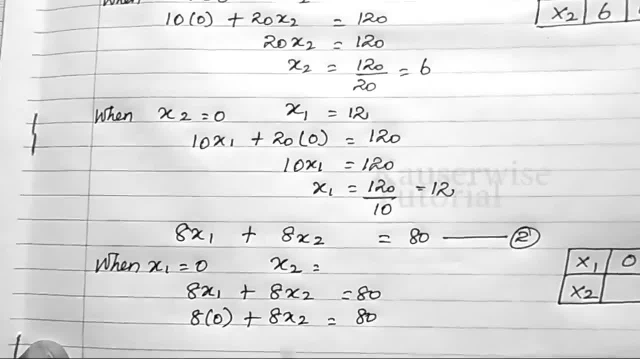 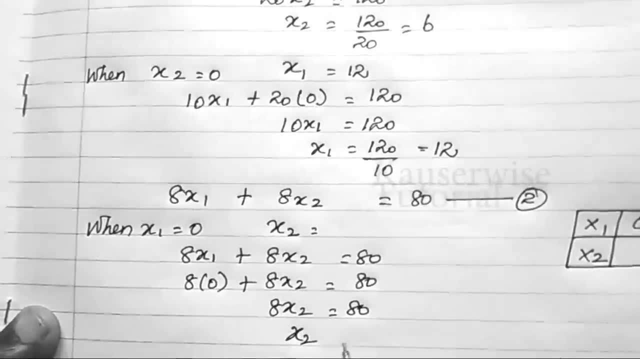 No Plus. 8x2 is equal to 80.. 8 into 0, 0. We have only 8x2.. 8x2 is equal to 80. So x2 is equal to 80 divided by 8.. 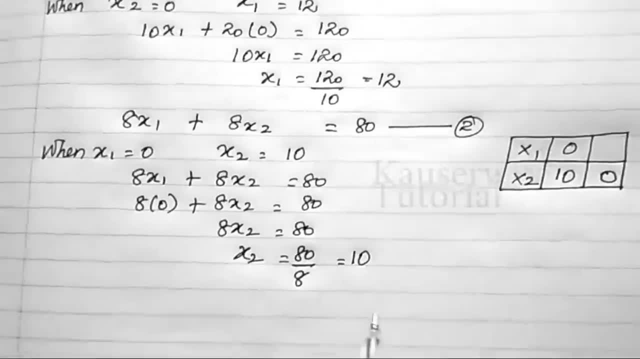 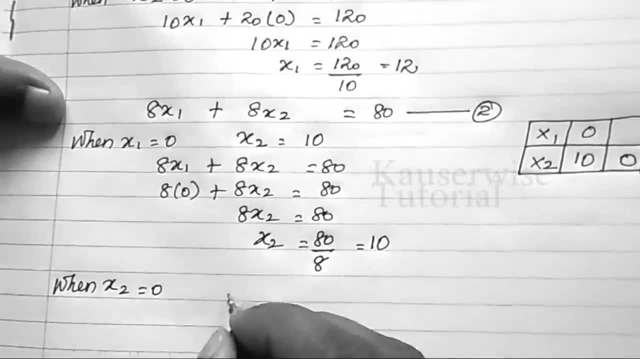 So what is the value? 10.. 10. In the same way, find the value for x1.. When x2 is equal to 0,, what is the value for x2? 8x1.. What is the equation? 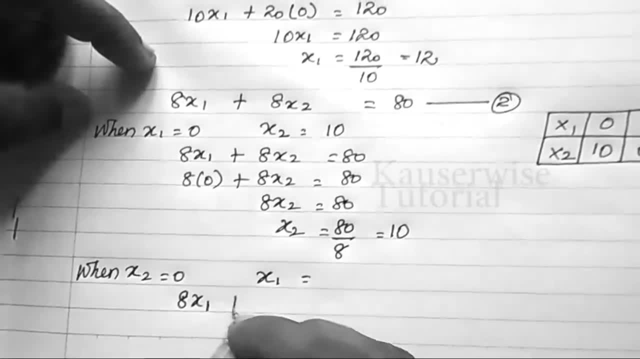 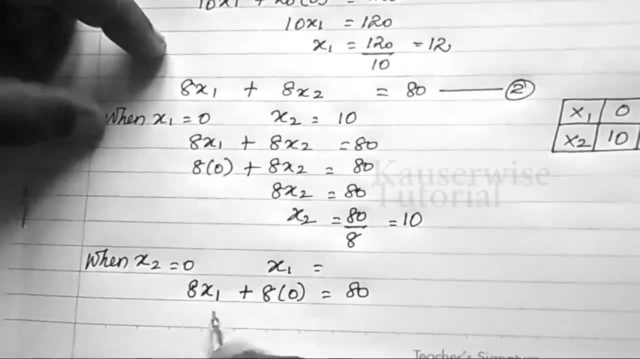 8x1.. No, So 8x1 plus 8x2 value is 0, is equal to 80.. 8 into 0, 0.. We have only 8x1.. 8x1 is equal to 80.. 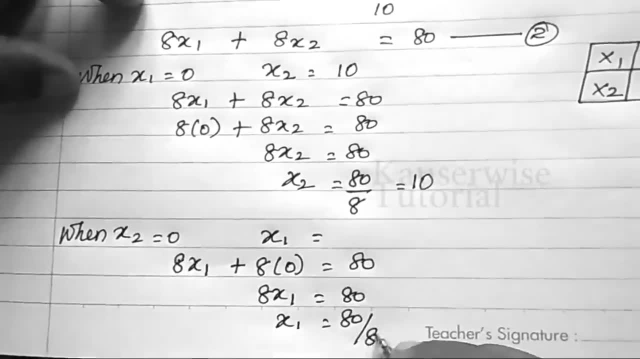 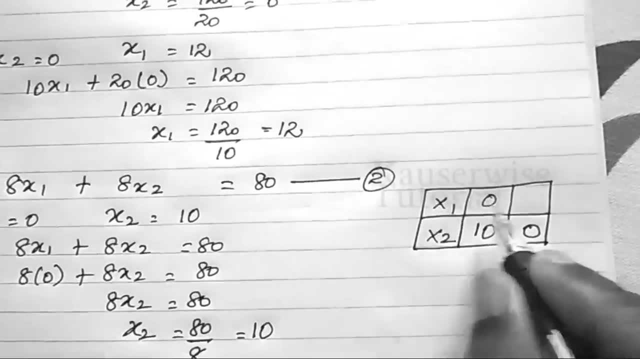 So x1 is equal to 80 divided by 8.. So value is 10.. So x1 is equal to 10.. When x2 is equal to 0, x1 value will be 10.. With this now, 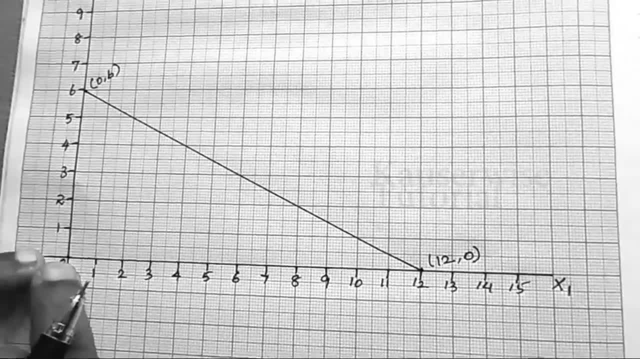 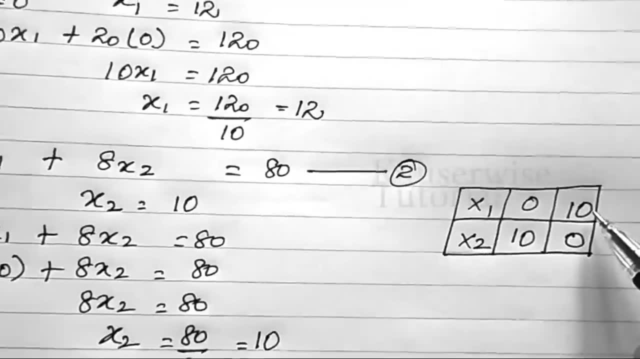 we can plot the second constraint: x1, 0, x2, 10.. This point: 0, 10.. Second one: x1, 10, x2, 0.. x1, 10, x2, 0. 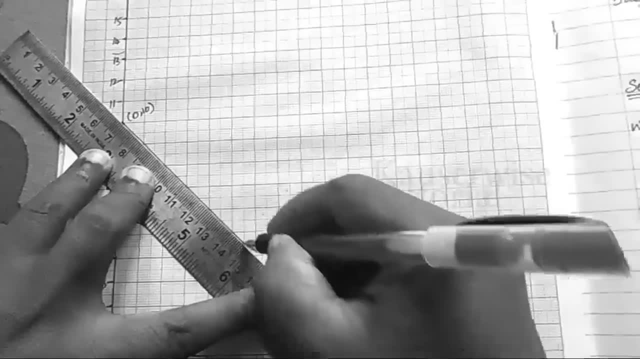 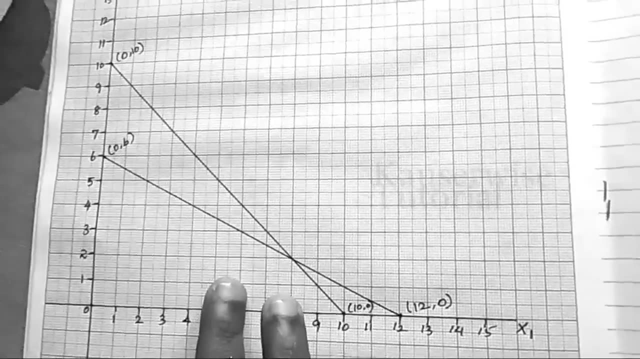 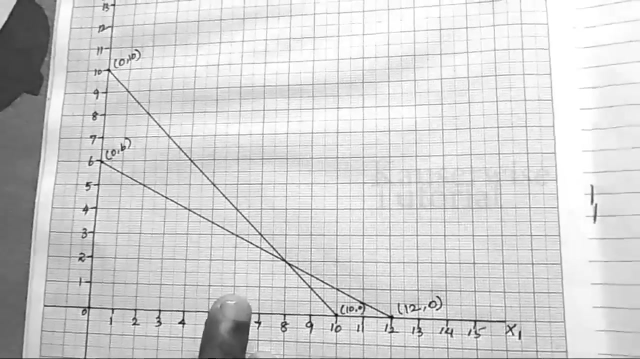 Now join the two points. This line represents the second constraint. Now you need to find the feasible region. In order to find the feasible region, just see the two constraints. That is two equation. Just check whether it is less than or equal to. 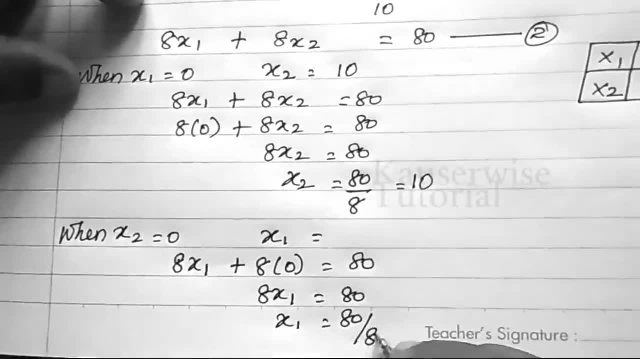 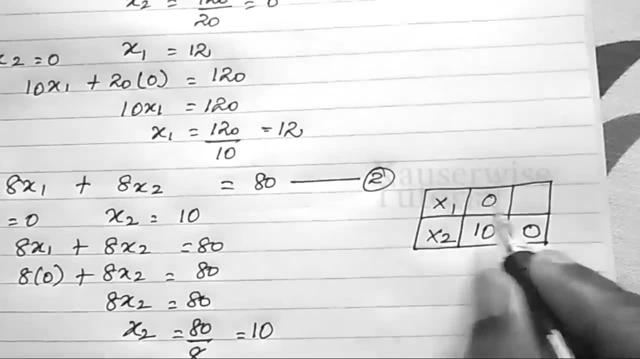 So x1 is equal to 80 divided by 8.. So value is 10.. So x1 is equal to 10.. When x2 is equal to 0, x1 value will be 10.. With this now we can plot the second constraint. 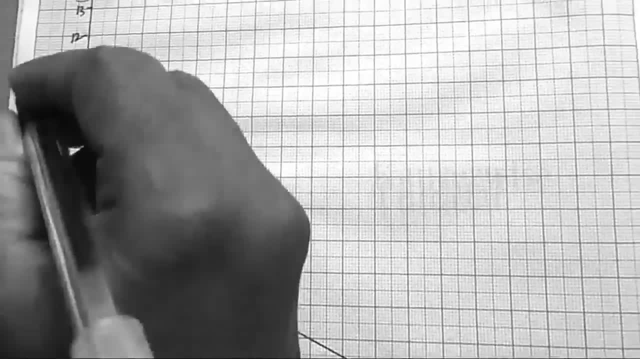 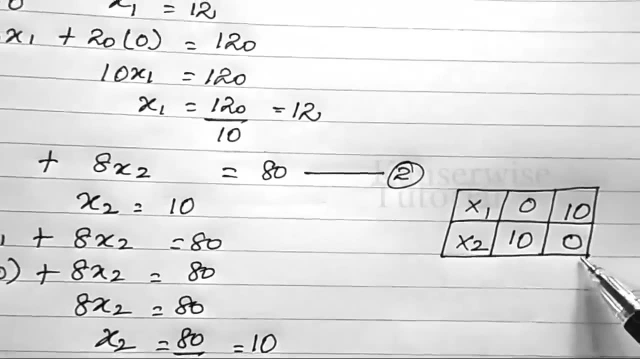 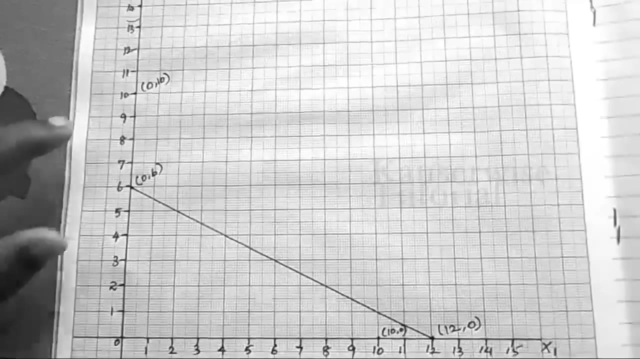 x1, 0, x2, 10.. This point: 0, 10.. Second one: x1, 10, x2, 0.. x1, 10, x2, 0.. Now join the two points. 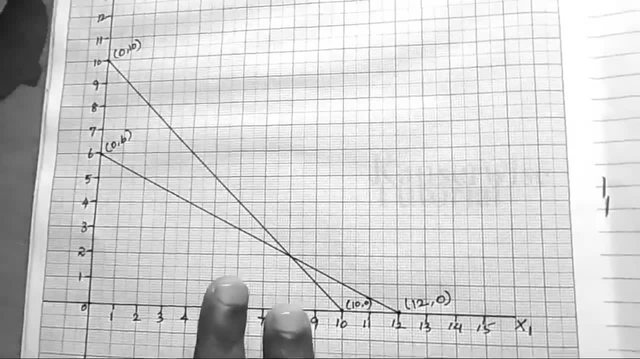 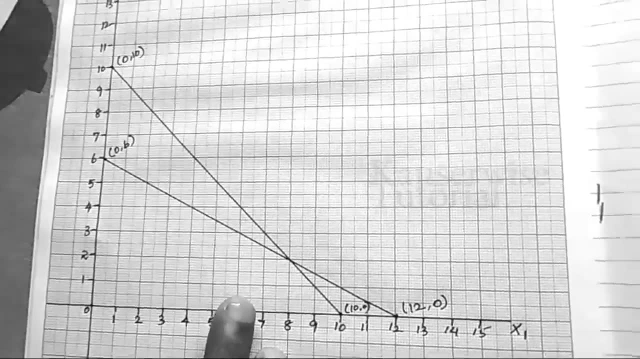 This line represents the second constraint. Now you need to find the feasible region. In order to find the feasible region, just see the two constraints, That is, two equations. Just check whether it is less than or equal to, or greater than or equal to. 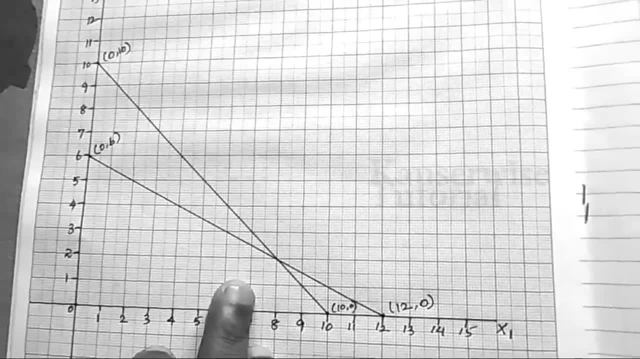 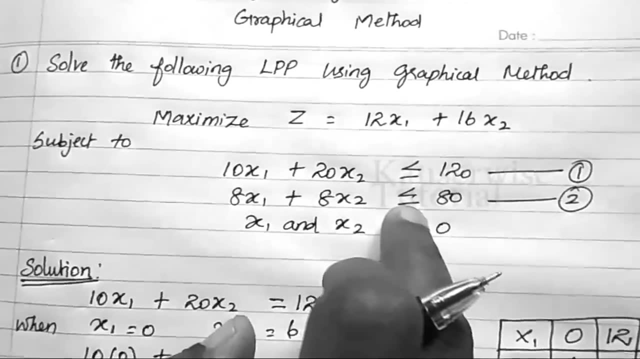 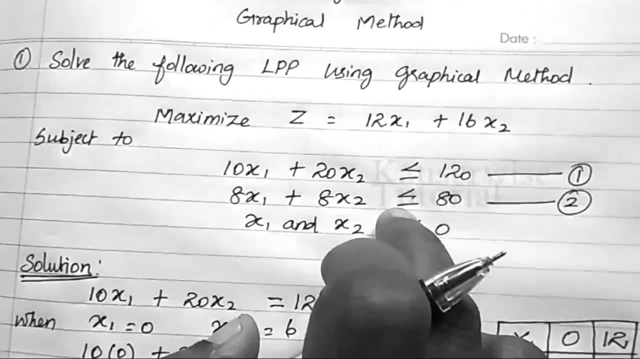 Because based on that only, you can able to find the feasible region. So look at the first constraint: Less than or equal to. Second constraint, also less than or equal to, Which means you have to find the feasible region. The feasible region should be below the line which you have drawn in the graph sheet. 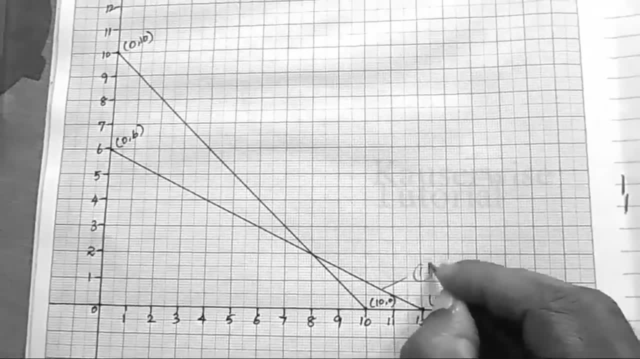 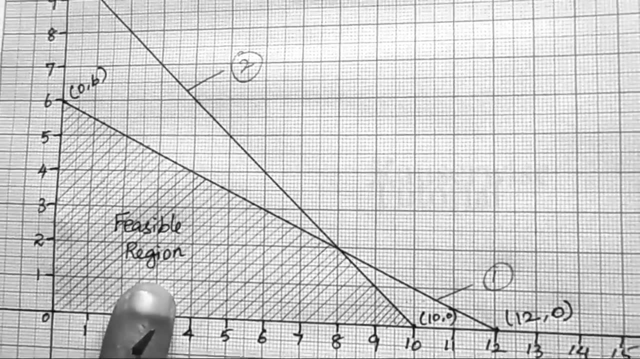 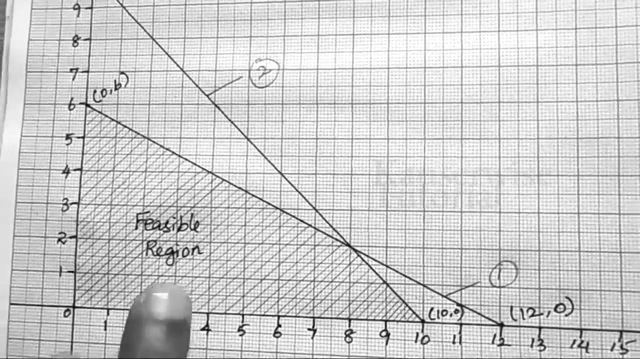 So this line represents the first constraint and this line represents the second constraint. See the shaded portion- is the feasible region. So in order to find the feasible region, both the constraints are less than or equal to, So the feasible region should be below the two lines. 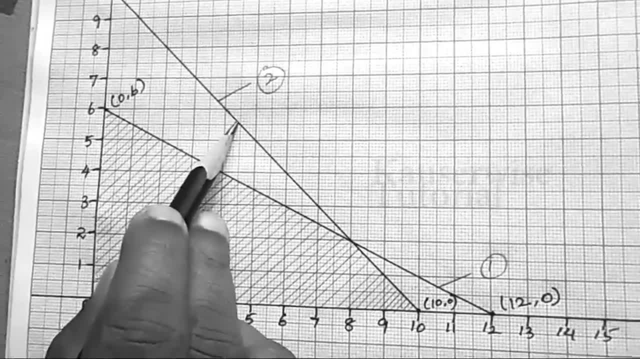 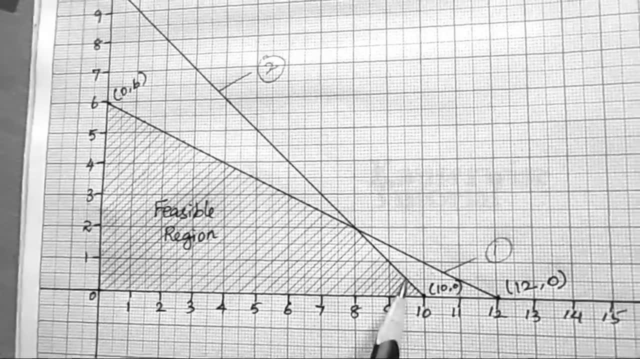 So if we select this one, this will be under second constraint, but above the first constraint. If we select this region, this will be under first. So this is the first region and above the second region. So these are the two regions, which is not feasible. 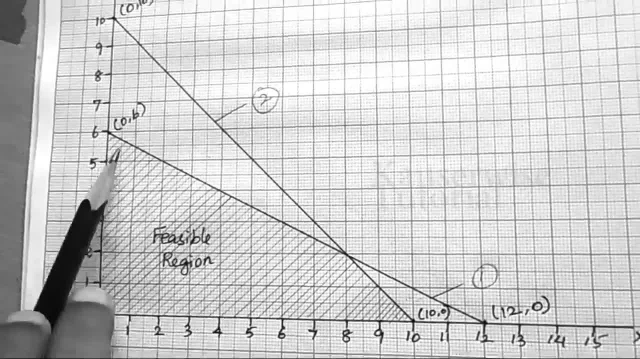 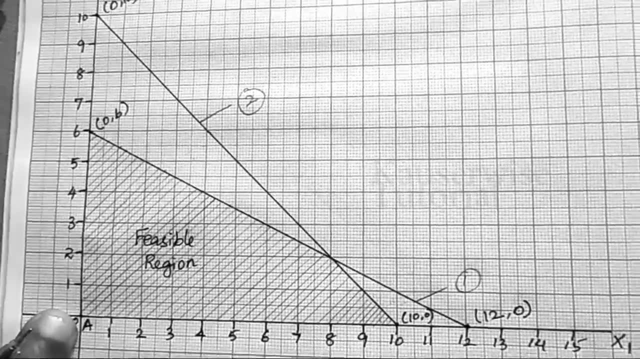 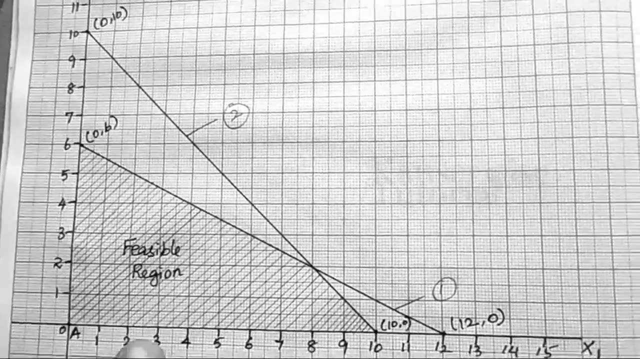 So this is the feasible region. Why? Because this particular shaded portion is below both the lines. We have four corners. This is the first corner, second corner, third corner, fourth corner. So these are the four corners in the feasible region. 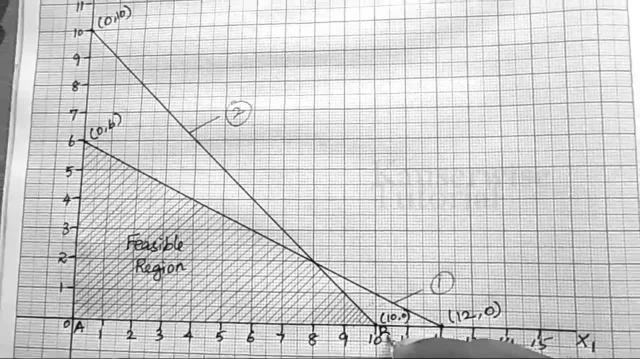 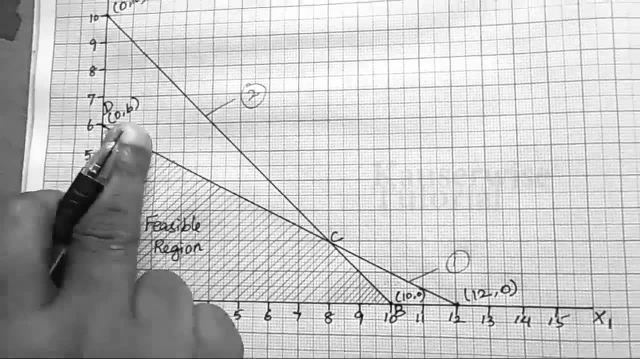 Now this will be A and this is B. This corner name is B, This is A, This is B, This is C And this one is D. The closed polygon- A, B, C, D- is the feasible region. So after finding the four points, so you have to find the value. 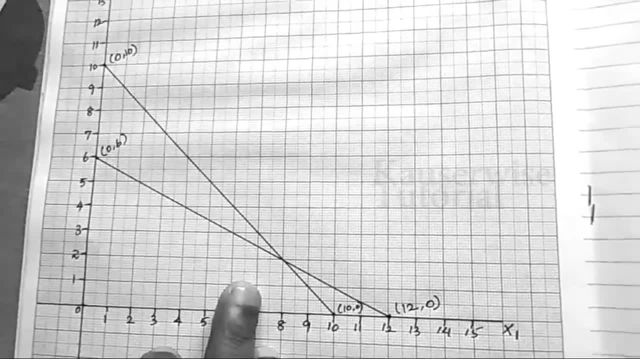 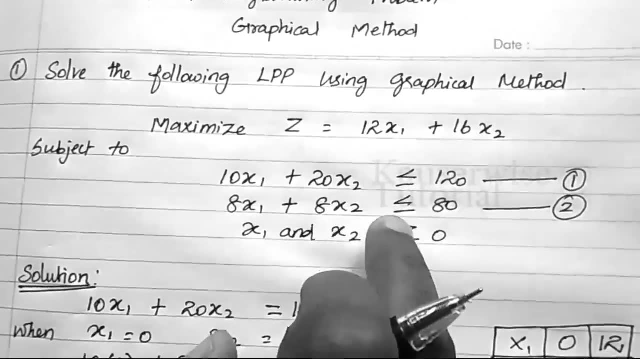 or greater than or equal to, Because based on that only you can able to find the feasible region. So look at the first constraint: Less than or equal to. Second constraint, also less than or equal to, Which means you have to find the feasible region. 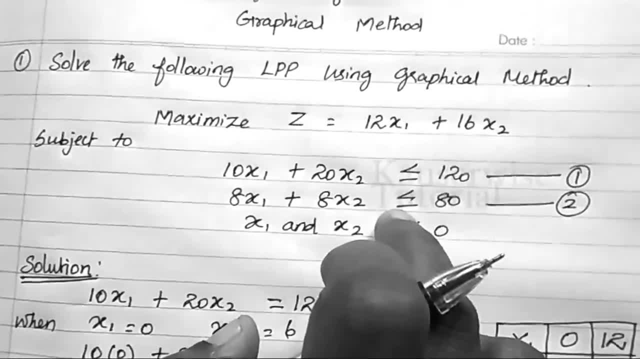 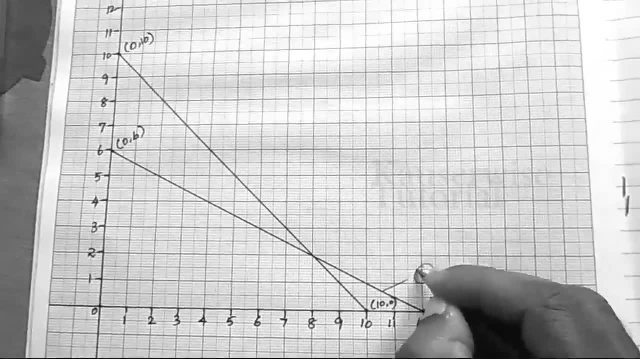 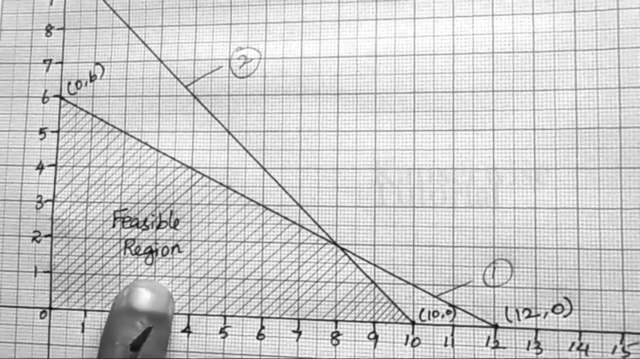 The feasible region should be below the line Which you have drawn in the graph sheet. So this line represent the first constraint And this line represent the second constraint. Okay, See, the shaded portion is the feasible region. Okay, So, in order to find the feasible region, 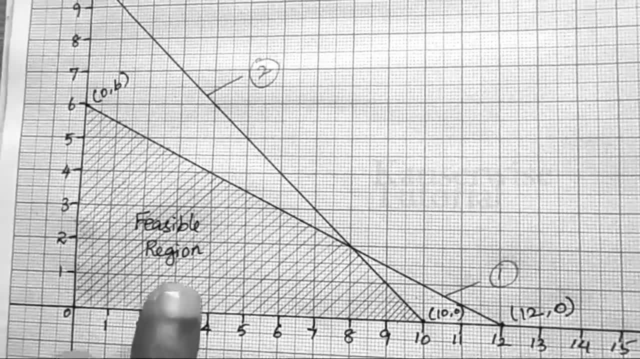 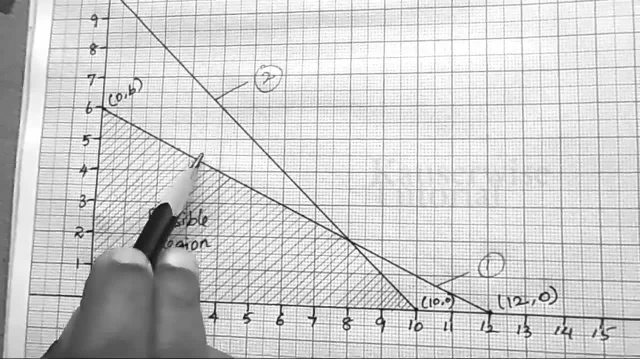 both the constraints are less than or equal to, So the feasible region should be below the two lines. So if we select this one, this will be under second constraint, But above the first constraint. If we select this region, this will be under first region. 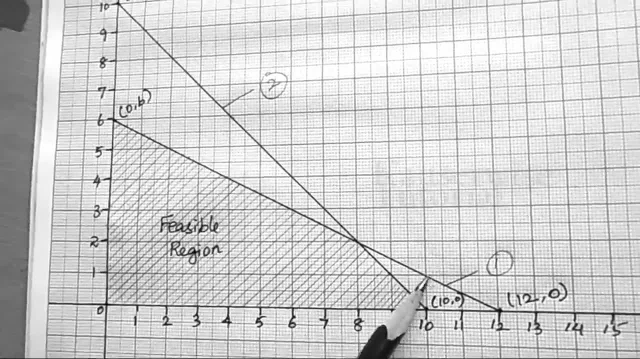 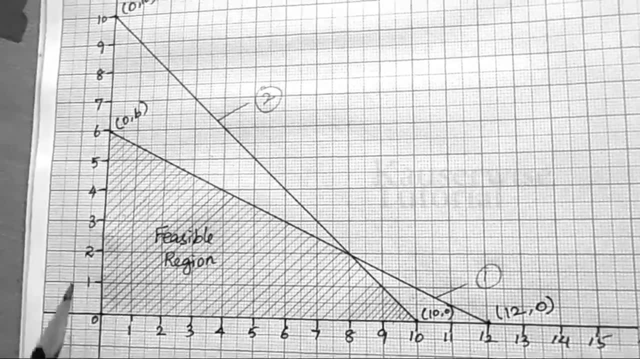 and above the second region. So these are the two regions. which is not feasible. So this is the feasible region. Why? Because this particular shaded portion is below both the lines. We have four corners. This is the first corner. 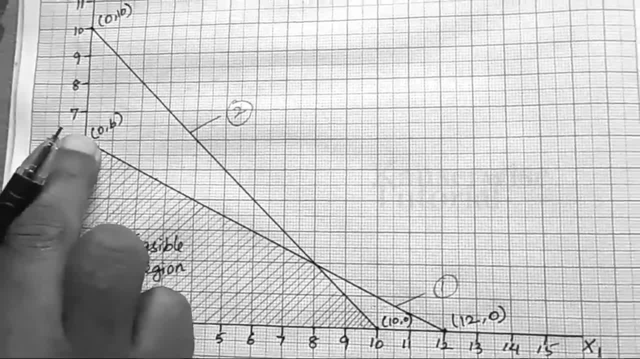 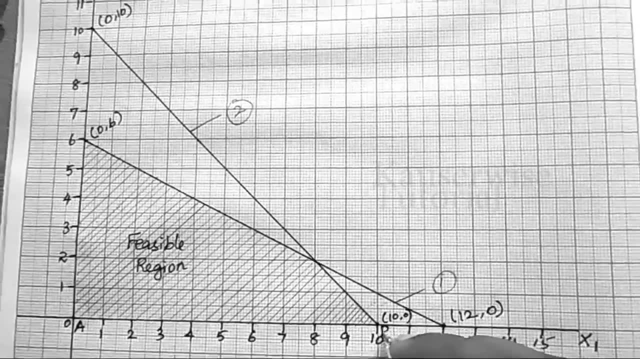 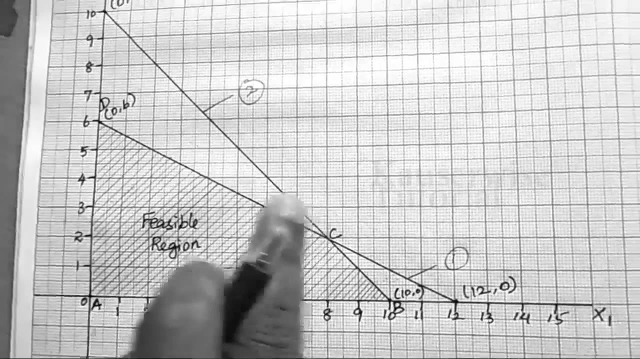 second corner, third corner, fourth corner. So these are the four corners in the feasible region. Now, this will be A And this is B. This corner name is B, This is C And this one is D. The closed polygon- A, B, C, D- is the feasible region. 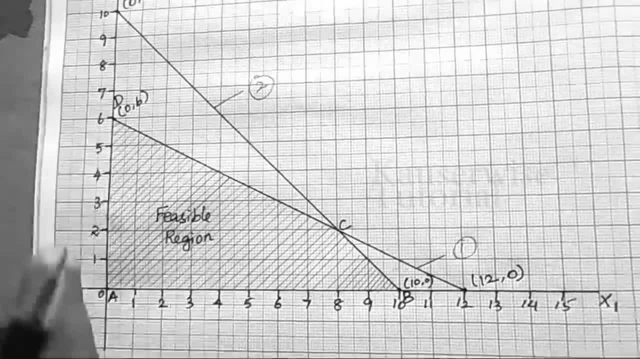 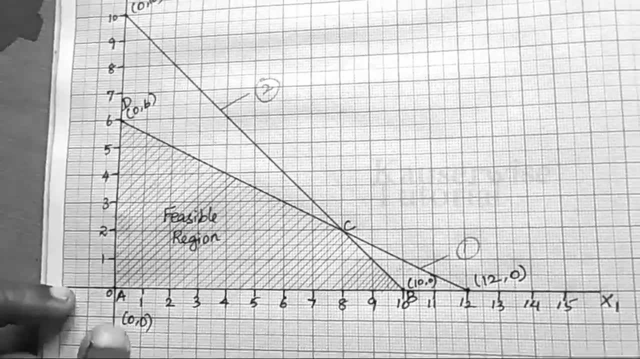 Okay, So after finding the four points- So you have to find the value- What is the value for A: 0 and 0.. X1 also 0.. X2 also 0.. What about B? B value is X1: 10,, X2: 0. 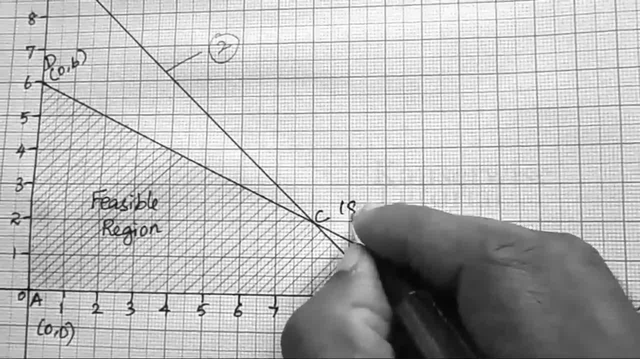 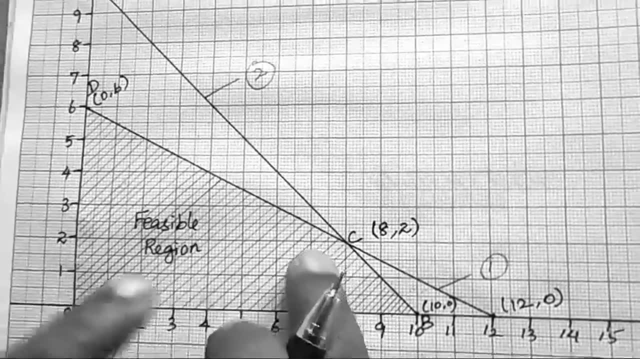 Look at the C point: X1, 8., X2, 2. X1, 8,, X2, 2. Just see 8 and 2.. Okay, In the same way, D D value. already is there: 0,, 6.. 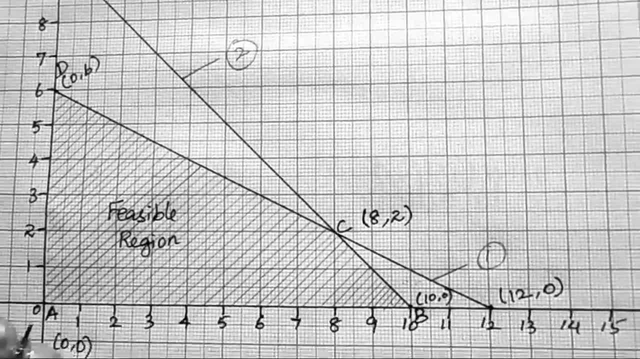 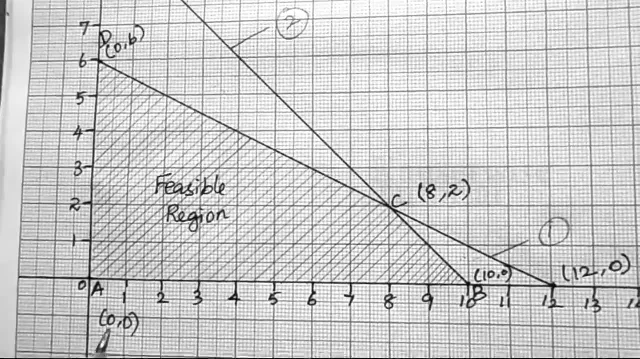 That is, X1 is 0.. X2 is 6.. So we have got four values for four corners. That is after finding the feasible region. Now we need to substitute these values in the objective function. What is our objective function? 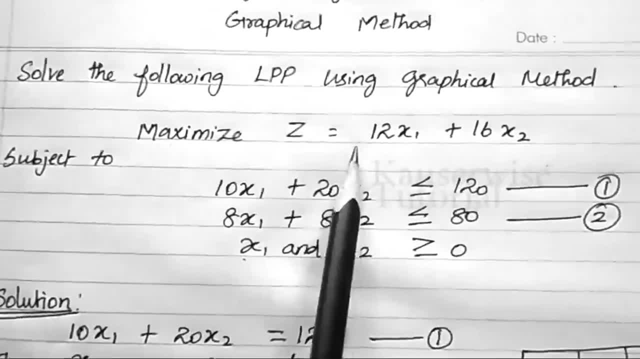 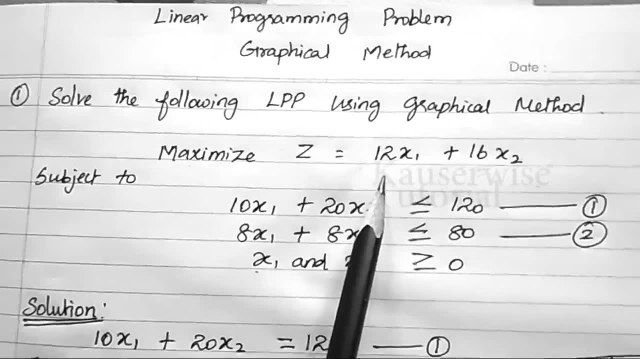 So this is the objective function, That is maximization. Z is equal to 12X1 plus 16X2.. So we have got four points now. So we have X1 value, X2 value in each points. 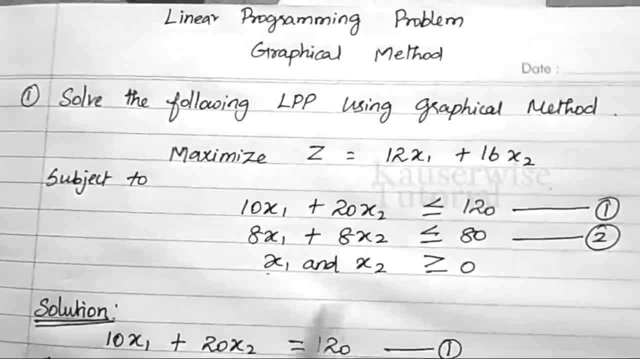 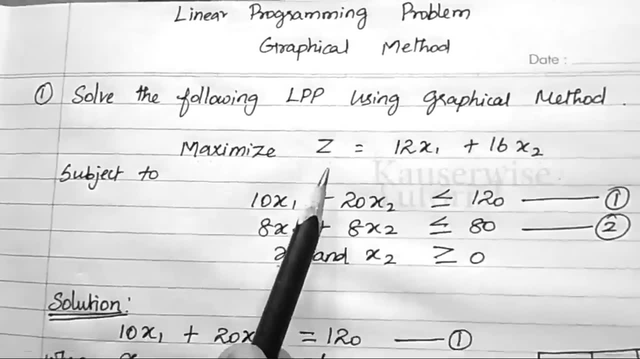 Okay. So now you need to substitute those values in this objective function in order to find the optimum point, That is, optimum corner. So let us see how I am going to work out this. See, Now I am going to substitute this value. 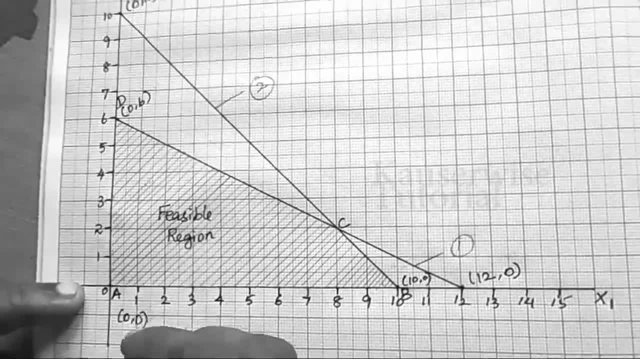 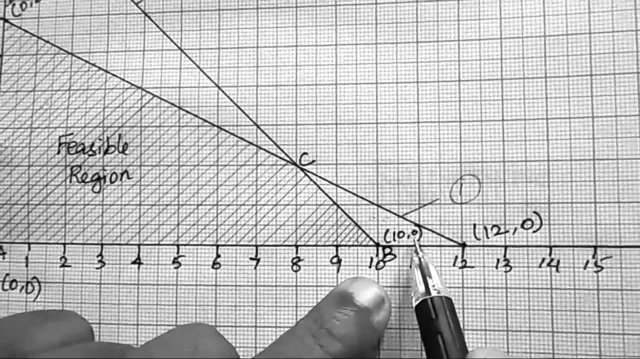 What is the value for A Zero and zero? X1 also zero, X2 also zero. What about B? B value is X1- 10, X2 zero. Look at the C point: X1, 8, X2, 2.. 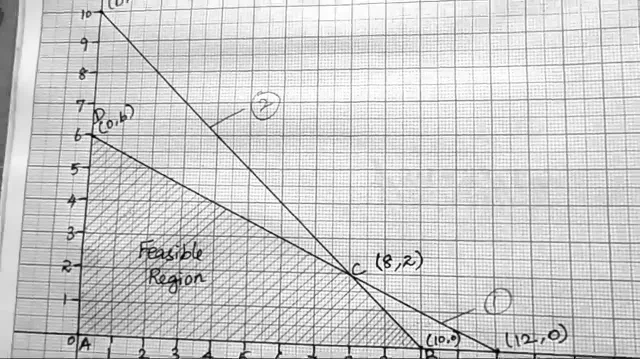 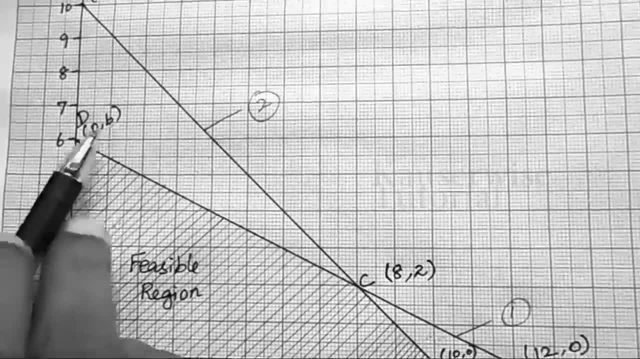 X1, 8,, X2, 2, just see 8 and 2,. okay, in the same way D, D value. already is there 0, 6.. That is, X1 is 0,, X2 is 6, so we have got four values for four corners. 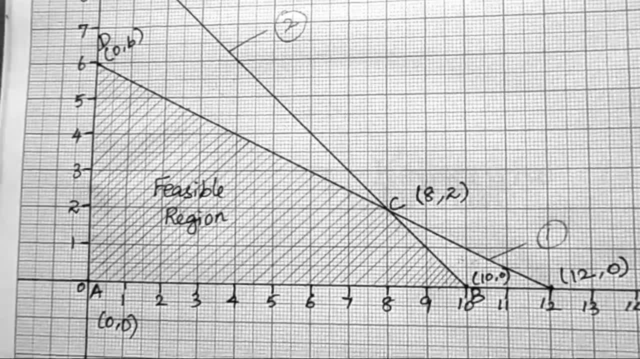 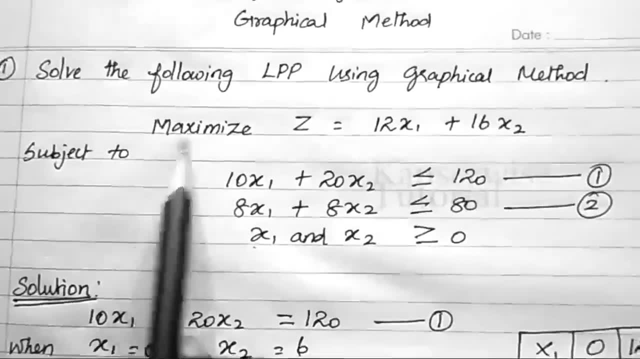 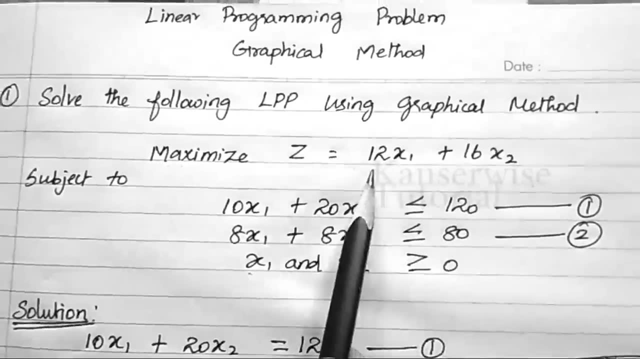 That is, after finding the feasible region. now we need to substitute these values in the objective function. What is our objective function? So this is the objective function. that is maximization. Z is equal. So we have got four points now. 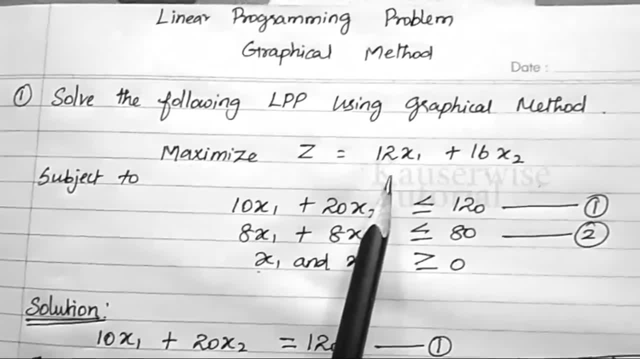 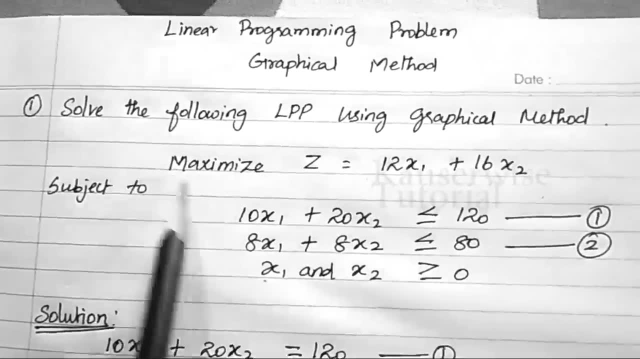 So we have X1 value, X2 value in each points. okay, So now you need to substitute those values in this objective function in order to find the optimum point, that is, optimum corner. So let us see how I am going to work out this. 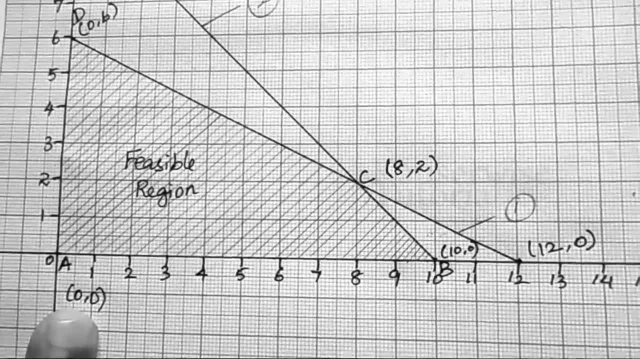 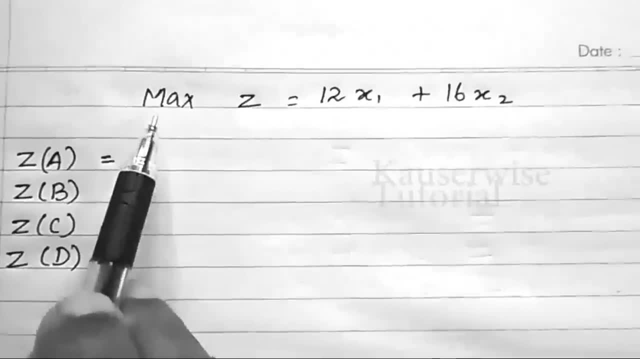 See, now I am going to substitute this value, that is, A's value. X1 value is 0, X2 value also 0. So now I am going to substitute, Substitute this value in the objective function. See, this is the objective function. 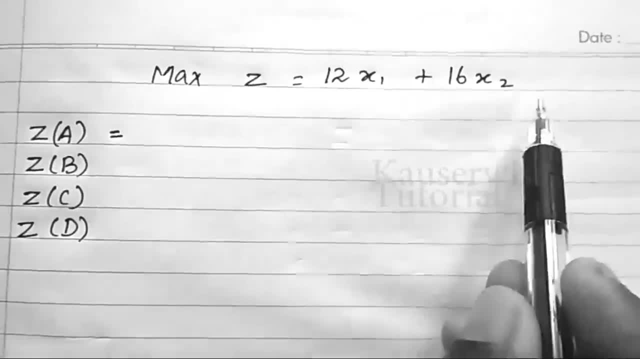 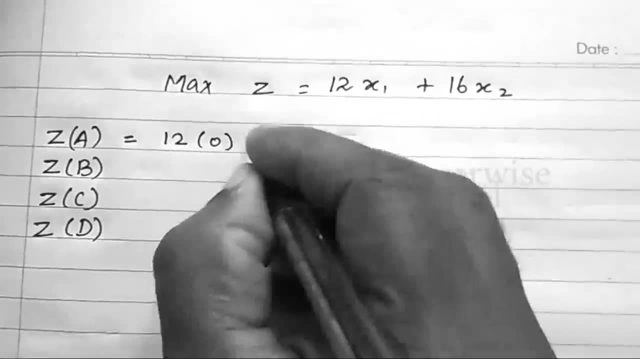 Maximization Z is equal to 12X1 plus 16X2.. So A's value 0, 0, no, So X1, 0.. 12, X1 value 0 plus 16, X2 value also 0. 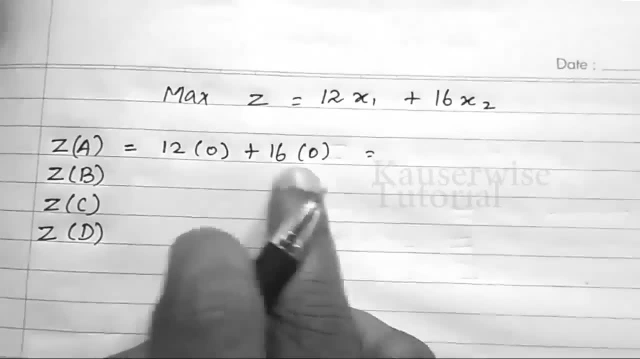 So what is the answer? 12 into 0, 0, plus 16 into 0, 0. So 0 plus 0, 0.. Then, in the same way, we need to find the value for B. 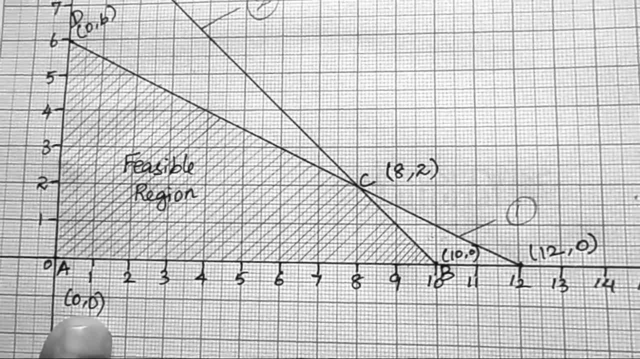 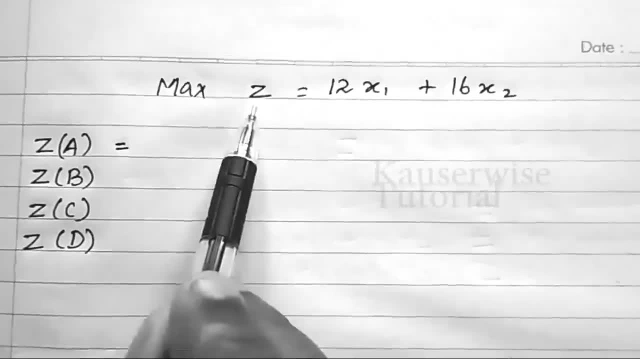 That is ace value. Ace value, X1 value is 0.. X2 value: also 0.. So now I am going to substitute this value in the objective function, See. This is the objective function. Maximization Z is equal to 12X1 plus 16X2.. 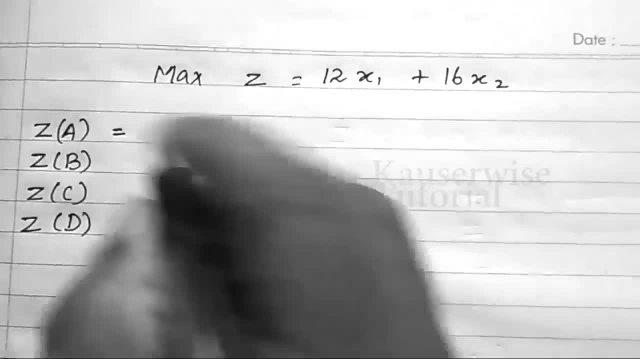 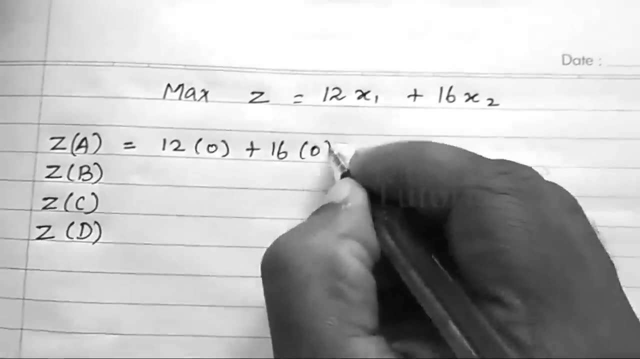 So ace value 0, 0.. No, So X1, 0.. 12.. X1 value 0 plus 16.. X2 value also 0.. So what is the answer? 12 into 0, 0 plus 16 into 0, 0.. 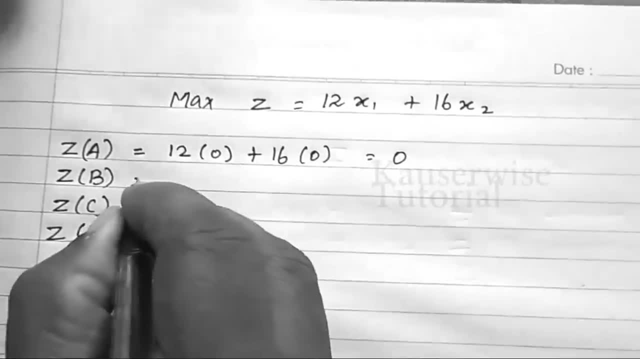 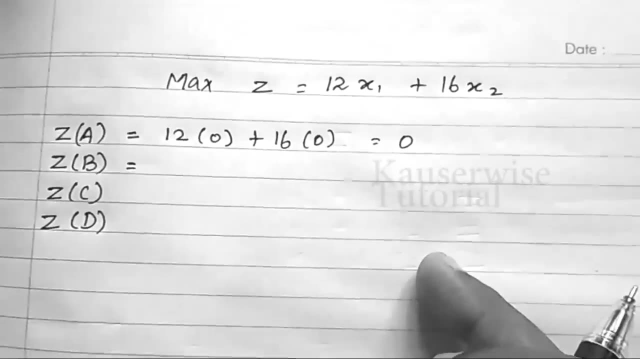 So 0 plus 0, 0.. Then, in the same way, we need to find the value for B, C and D also. in order to find the optimum point, Look at the Bs X1, X2 value 10, 0.. 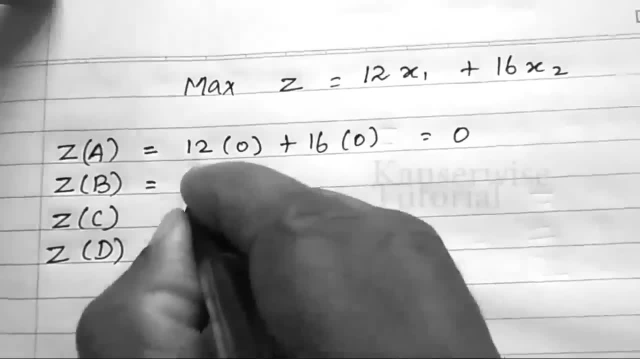 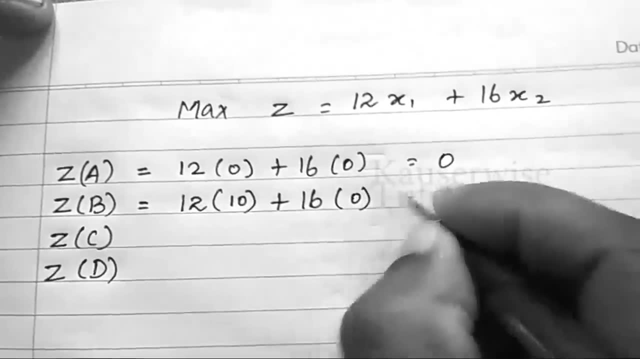 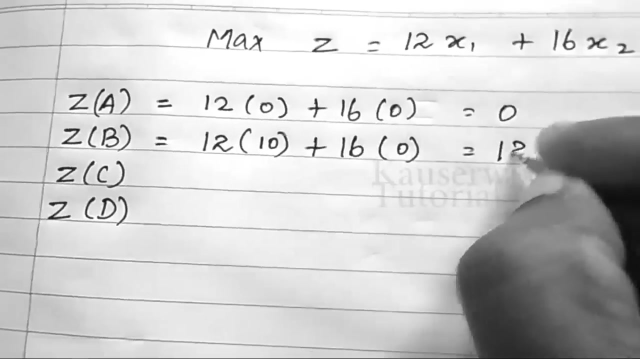 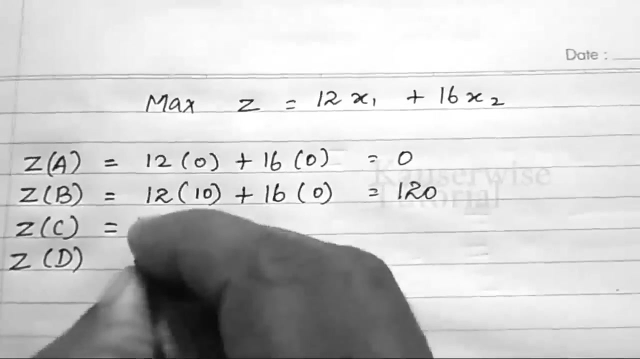 X1 value 10,, X2 value 0.. So 12X1 value 10 plus 16X2 value 0.. So 12 into 10,, 120 plus 16 into 0, 0.. 0.. 120.. A- B is over. Now look at the C. X1 is 8.. X2 is 2.. For C: 12. X1 is 8 plus 16.. X2 is 2.. 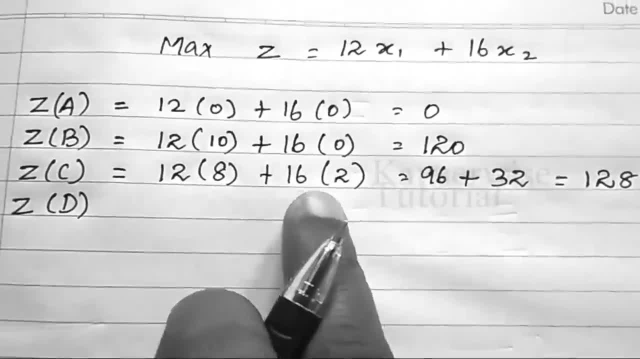 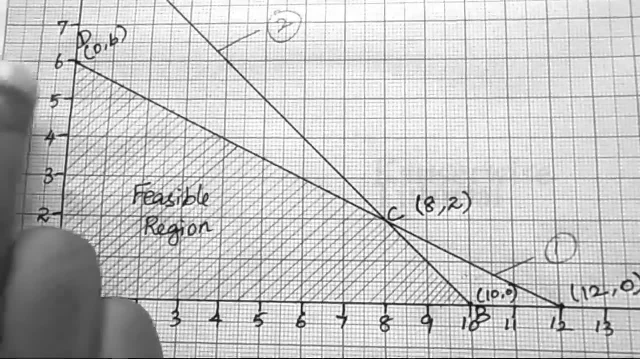 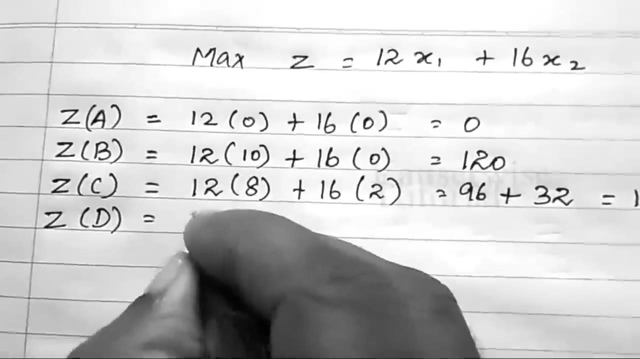 12 into 8,, 96 plus 16 into 2,, 32.. So 96 plus 32 is equal to 128.. A B C's are over. Now look at the fourth one, D. D's value is X1. value is 0.. X2 value is 6.. For D: 12.. X1 value is 0 plus 16.. 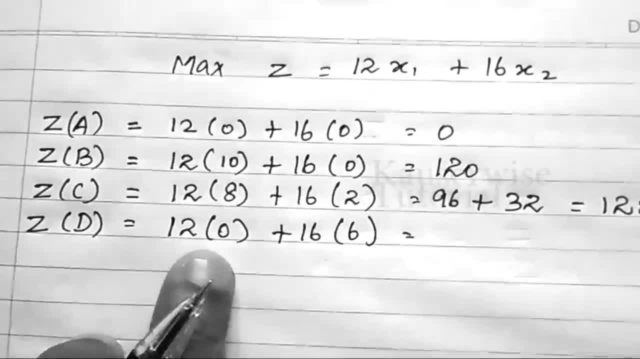 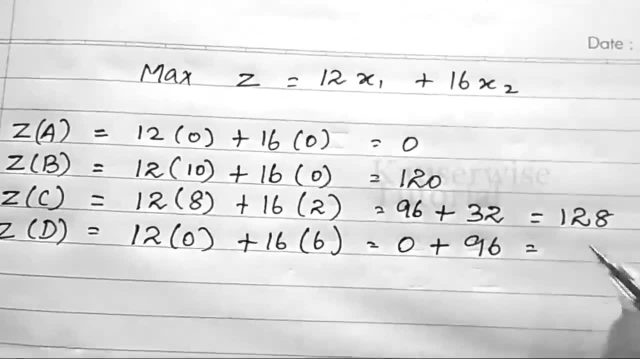 X2 value is 6. 12 into 0, 0, plus 16 into 6, 96. So 0 plus 96, 96.. Now we have got the Z value for A, B, C, D, Since it is a maximization problem. 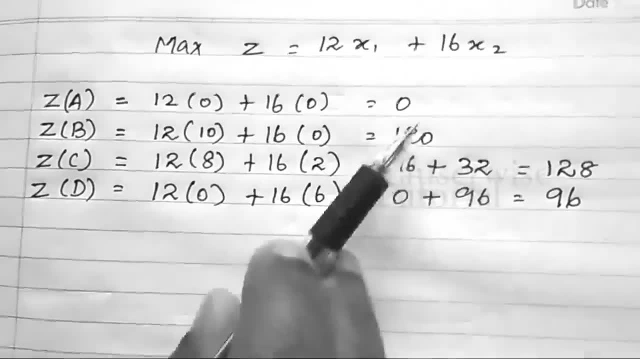 we need to find the Z value for A, B, C, D. So we need to find the Z value for A, B, C, D, The maximum point. So look at the four answers. Which one is highest value? 0,, 120,, 128,, 96. So. 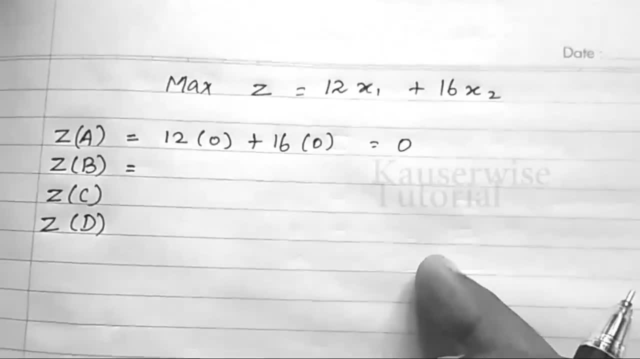 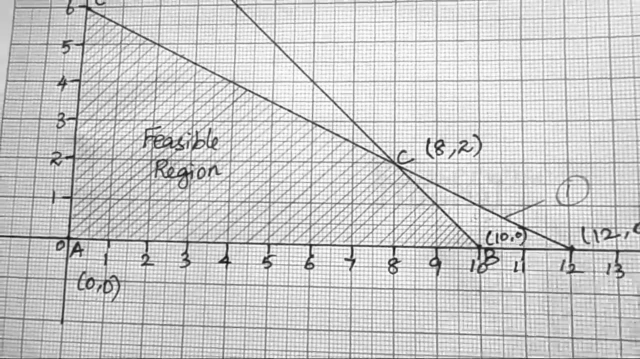 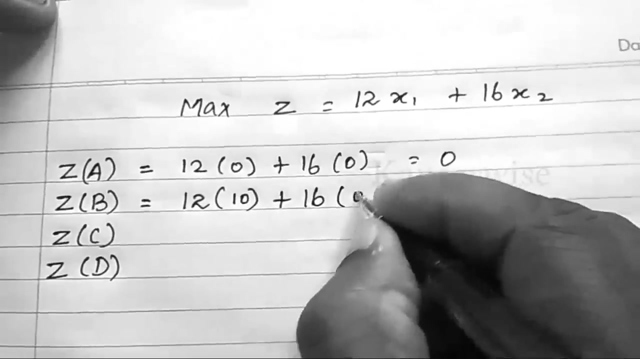 And D also. in order to find the optimum point, Look at the B's X1, X2 value 10, 0.. X1 value 10, X2 value: 0.. So 12, X1 value 10 plus 16, X2 value 0..